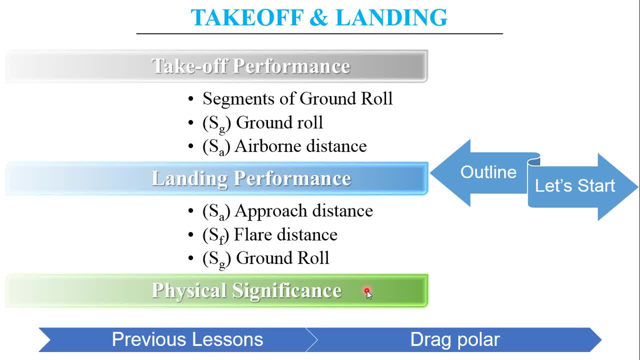 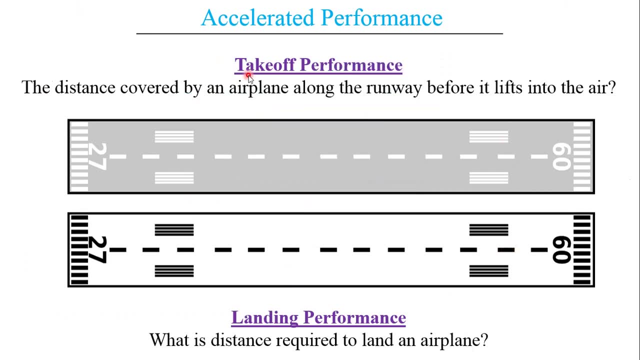 And finally, we will be discussing about the technical significance of takeoff and landing and the need for measuring or calculating the distances. Let's get started. So, takeoff and landing, the performance of these both are categorized under the accelerated performances. So in both these topics, acceleration is playing some part, because during takeoff, the aircraft is starting from velocity. 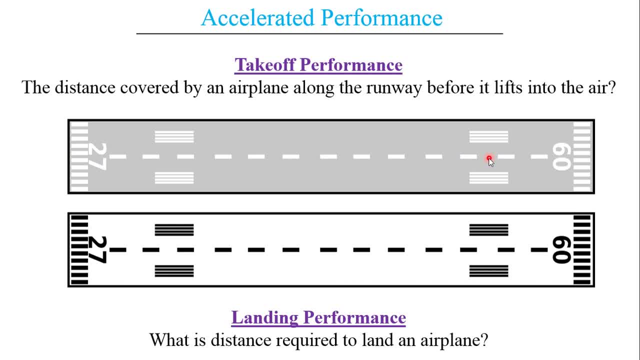 And it is accelerating to some particular velocity and it is taking off from the runway And similarly, in the case of landing, the aircraft which was being accelerated is decelerated down and it is brought to rest. That is a zero velocity. So what is that we are dealing with here? and takeoff performance. 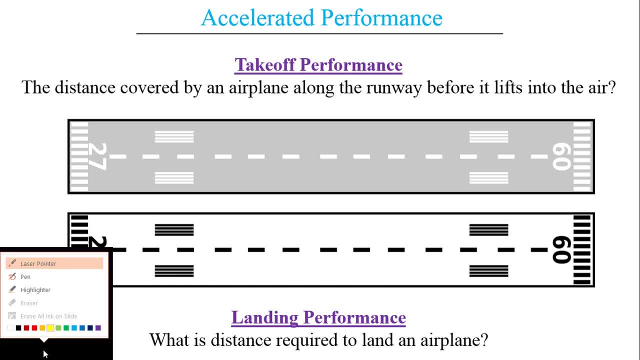 The main question which we Will be answering is that the distance covered by an airplane along the runway before it lifts off into the air. So we will be, in particular, focusing on this distance and trying to calculate this distance, And this makes a pretty much important topic in the landing performance. 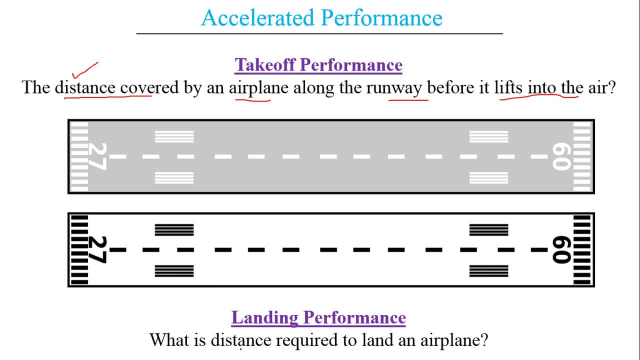 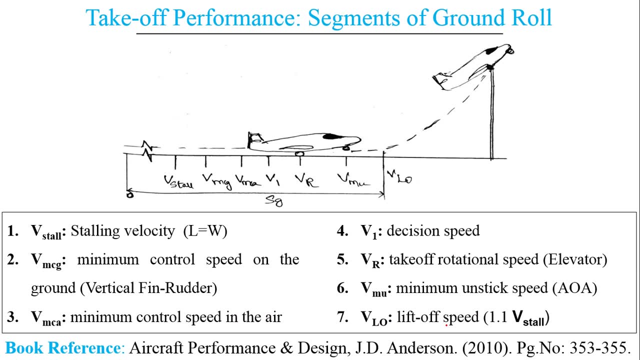 We will be concerned about the same distance which is required to land. So landing performance can be considered as the reverse of takeoff performance Now. So here, when we get into takeoff performance, the takeoff performances ground role. this is the signifies. ground role can be divided into many different segments. 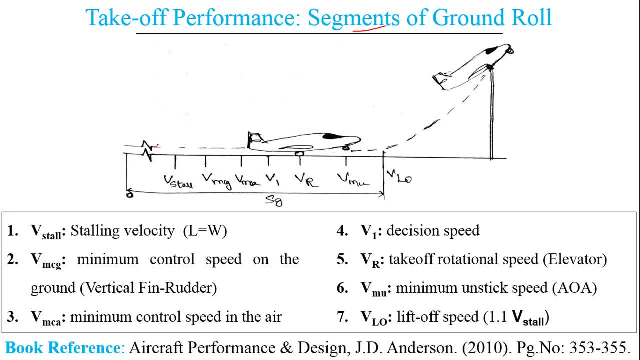 So these segments include the velocity which The aircraft achieve during the It's takeoff. So at first let us consider that aircraft is at 0 velocity and ah, With sometimes and distance, I mean velocity gets accelerated, So the velocity gets increased to a velocity known as. 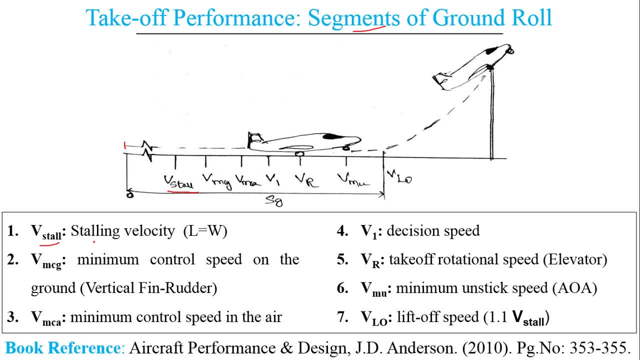 We stall, So we should, is nothing but the starting velocity. starting velocity is the turning velocity On the minimum velocity which is required For light countries. Thanks, Reg. towers a message for an aircraft to stay airborne and in the case of stalling velocity, the lift equals the weight. 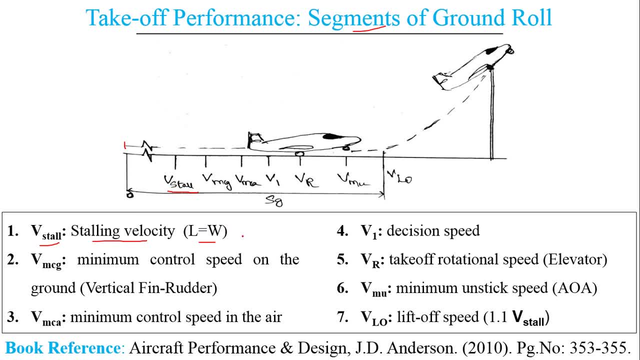 of an aircraft, but still, in this case the lift off isn't achieved as lift is equal to weight, which is the cruise condition. so takeoff condition: we need lift greater than weight. okay, this is the lift. and if the lift is greater than the weight which is pulling the aircraft downwards, the aircraft gets. 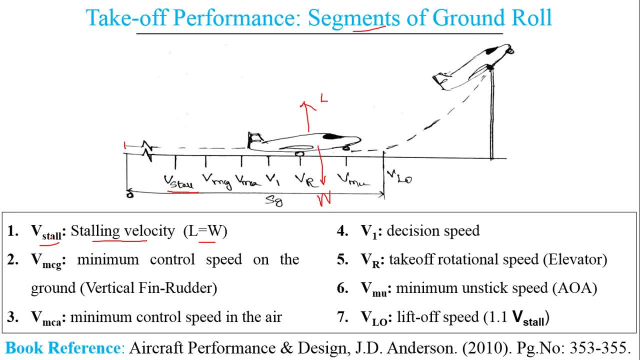 lifted off or taken off. next, when the aircraft further accelerate, the aircraft achieves the speed bmcg, which is the short form of minimum control speed on ground. so basically, when we talk about aircrafts, we pretty much talk about the control surfaces, such as rudder elevator. 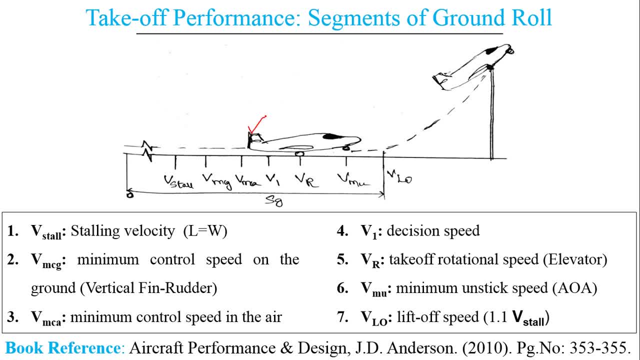 flaps and everything. but one common thing to be noted over here is that all these control surfaces, may either it be primary, secondary or tertiary, they are dependent on aerodynamic forces to operate. so if we want the rudder to operate, such as if we deflect the 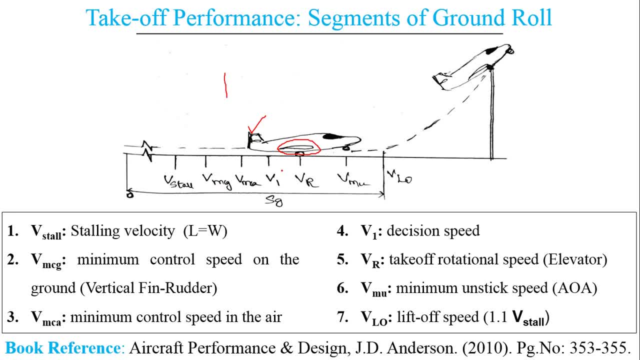 rudder, left or right, we need the aircraft to yaw. but how does it happen in order for this to happen? because when the aircraft is at rest, this is impossible because rudder cannot be operating as it does not operate on the aircraft, so we need to operate the aircraft on the aircraft. 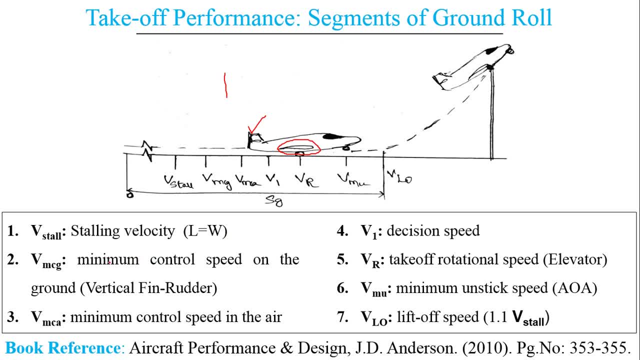 uh, match its minimum requirement. so here we need some velocity at which these, all these control surfaces become functional. so this particular velocity is known as yeah, vmcg. so further, at this point we know that as the control surfaces are active, that is, they can be accessed, so the aircraft can be controlled and in case of 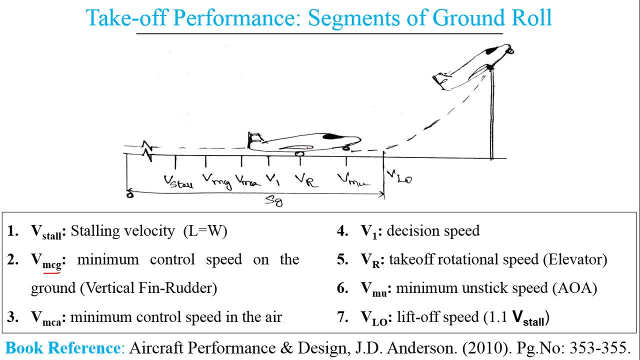 engine failure, the rudder is easily used and the aircraft is stabilized. now vmca is nothing but the vmcg. that is a minimum control speed on ground which is translated to the air. consider that aircraft has taken off and at that point the there is no contact between the ground and an f. 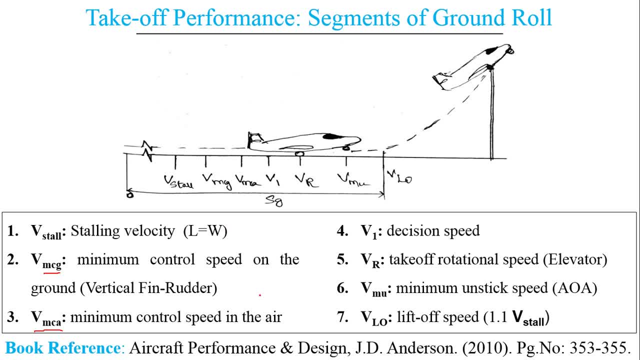 so, when this condition achieved, the speed or velocity at which the aircraft can be controlled, or the airplane can be controlled, is known as the minimum control speed on air. Similarly, the aircraft proceeds to the V1, so this is an important speed, the decision speed. so at this speed the airplanes pilot decides whether to take off or to abort. 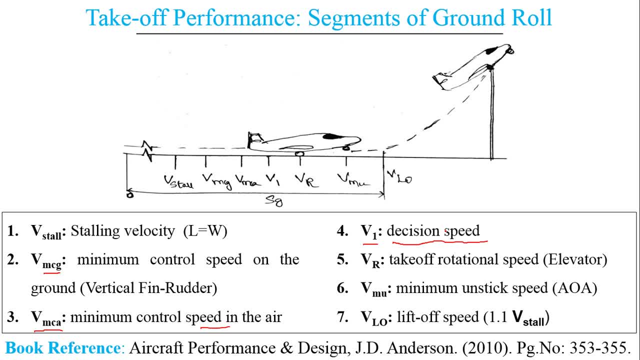 So in case of engine failure before this speed, the pilot will abort the take off and in case of engine failure after this speed is achieved, the aircraft can perform a take off and it will come back and land. So we have been quite commonly talking about speed and velocity interchangeably. 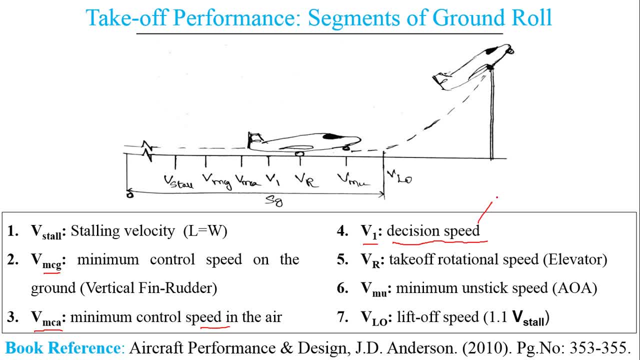 What is the difference? Speed is nothing but same as velocity. Still, Speed is a scalar quantity, as it does not have a direction component in it, and velocity is a vector quantity, as it has a direction component in it. So, in common, both are one and the same. 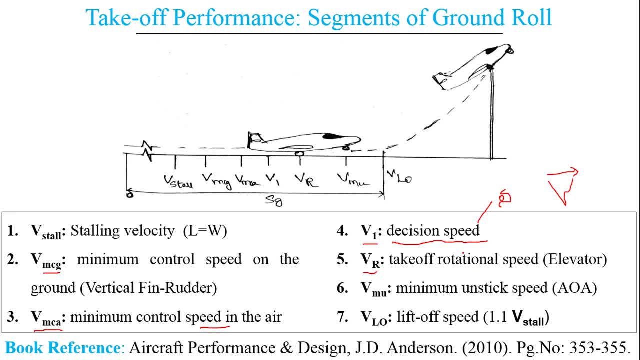 So when aircraft, weather increases its velocity, so a particular velocity is achieved, the Vr, so it is a take off rotational speed velocity. So in this is the velocity, So in this is the velocity, The velocity at which the elevator is deflected in order to provide an increased angle of 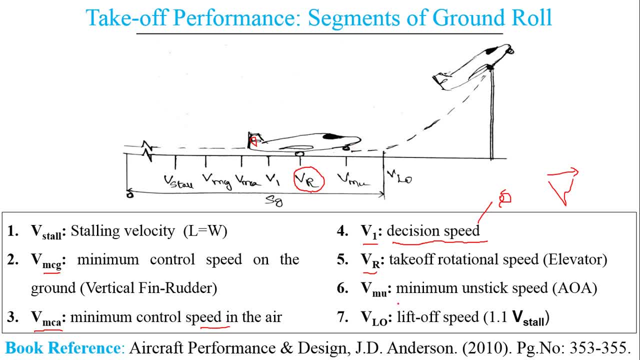 attack or generate the lift off. So when the aircraft further accelerates, so it has a point where the wheel or tyre of an aircraft lifts off the runway and the contact is lost. So At this point The velocity at which this is achieved is known as the minimum unstake speed. 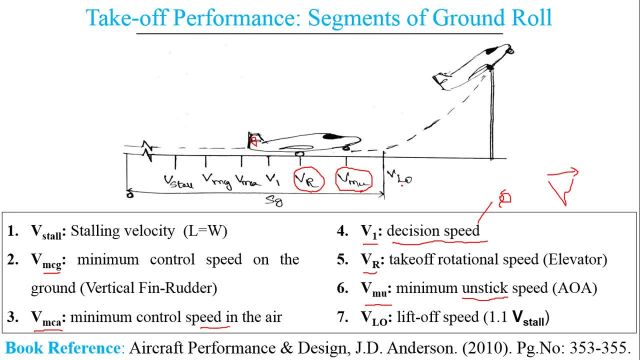 So here the aircraft further proceeds to the lift off velocity, so it is somewhat greater than the Vmu and Vr. This is particularly for safety purposes and the Vmca is basically for reference purposes. Another point to note is that The velocity of lift off 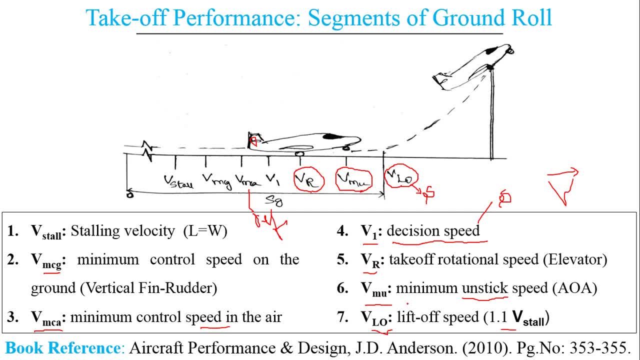 Is 1.1 times the velocity. stall result: stalling velocity. This point 1 difference is a segmented into these many segments. For further details you can refer the book contents. so this particular topic is dealing with the page number 353 to 355.. 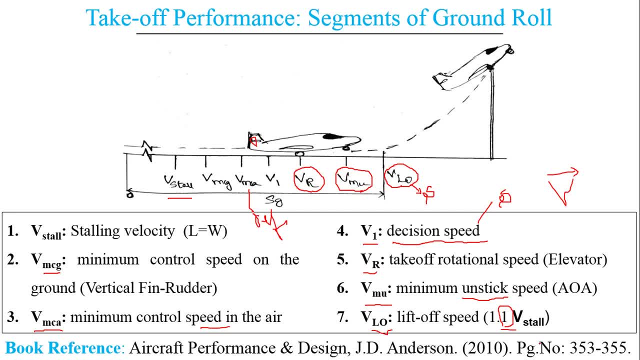 And with respect to 269, this particular topic is dealing with the page number 353 to 355.. So, As a result, the velocity is better. So this particular topic is dealing with the page number 352 to 355.. So the velocity of lift off. 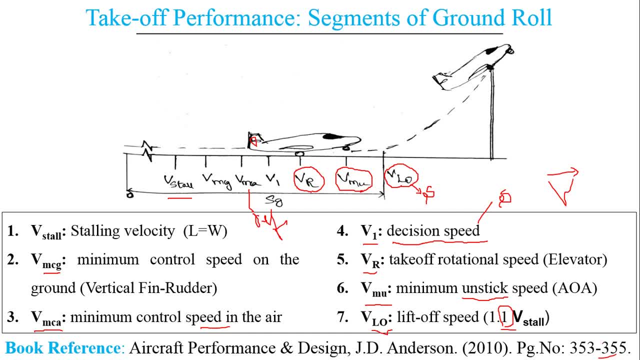 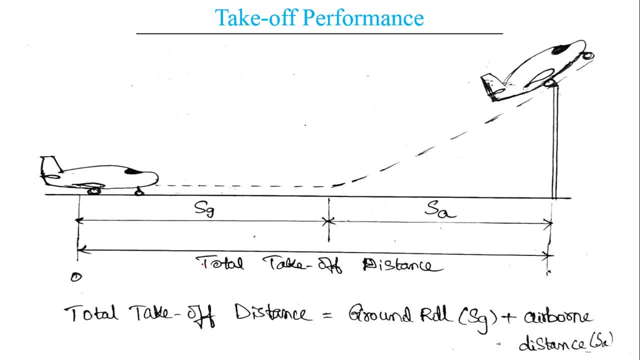 355 of airplane performance and design. so here now let's get into the takeoff performance. as I said, according to the federal aviation regulation, so this is a body which decides the rules and regulations for operating an aircraft and designing an aircraft, of course. so let us consider a scenario of takeoff. so 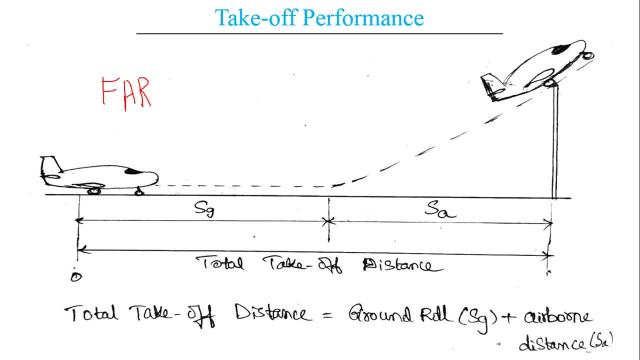 the aircraft is going to start from a position where the velocity is zero and it is going to accelerate to some velocity and further acceleration will cause it to lift off, as the lift is generated from the wing and the aircraft is going to lift off and climb into the air and, according to this, 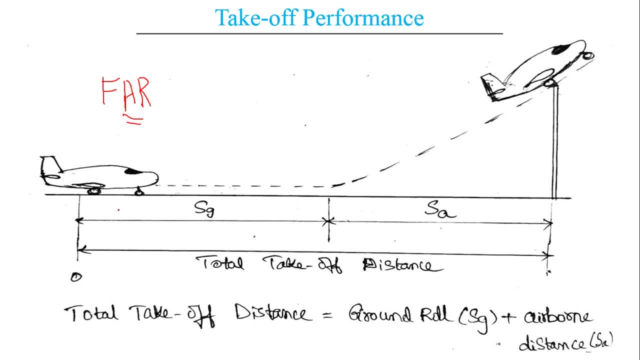 regulations rule. the aircraft must also accelerate and lift off from the runway. similarly, it also needs to achieve or cover an additional obstacle height, that is, the FF needs to clear this obstacle height. so this is known as a HOV. so this is the obstacle height. they have pretty much decided. this particular value can. 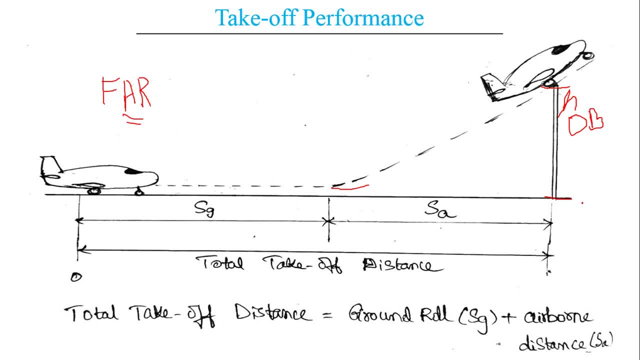 be either 35 feet or 55 feet, the on the type of the aircraft. so an aircraft or airplane in particular needs to clear this obstacle height in order to consider it as taken off from the runway. so for this case, the takeoff distance can be divided into two particular portions, that is, the ground roll sg and the 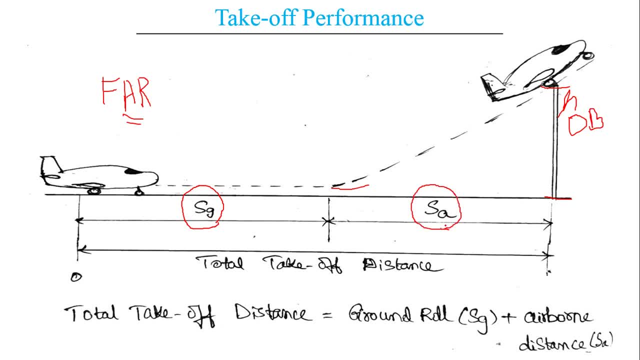 distance at which it is airborne during its clearing- the obstacle height. so this is known as the airborne distance. that so the total takeoff distance is a summation of ground roll distances g and airborne distance sa. now we will be deriving these both values separately and we will be 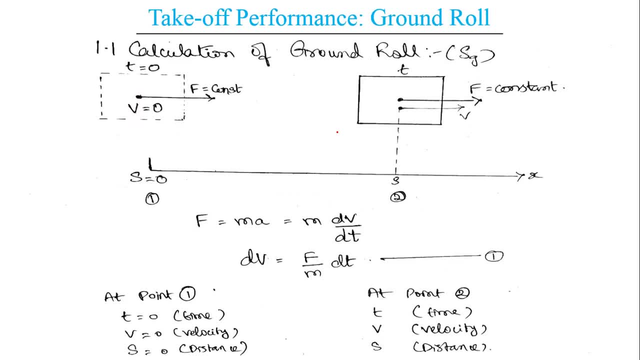 adding those in order to find the takeoff height distance. so here let's calculate the ground roll. when we are considered with the ground rule, the aircraft is still on the ground and we can basically bring it down to the physics in order to derive this. so let us consider a mass particular 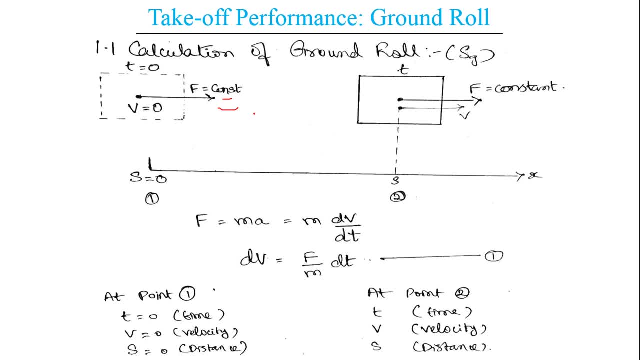 mass of a body and our constant force is acting on it. and let us take the initial conditions as, at time zero, the velocity is v equal to zero and the distance is also zero. so this is at reference point one, and we are considering another point two at which the airplane has 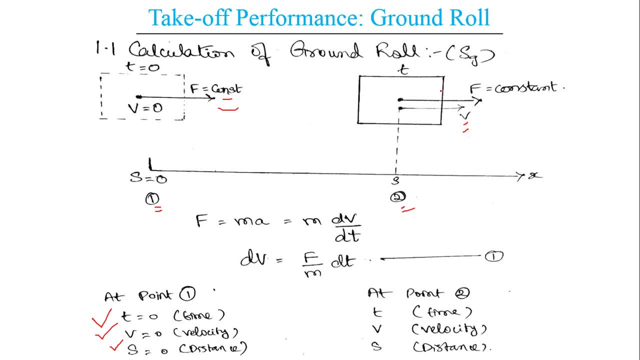 an increased velocity v, the force is constant and the time is also increased as the time taken from starting from this point to the point two, where the velocity is increased to v and the distance is also increased from s equal to zero to some particular distance. so when we bring the 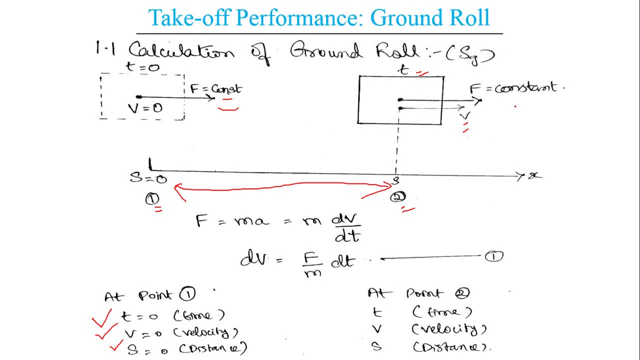 force down to physics, we can easily derive it as a force is constant, from newton's law we can write: as force is mass times, acceleration. so here, acceleration. we know that acceleration is nothing but the change in velocity, right, change in time. so here, when we rearrange this equation, 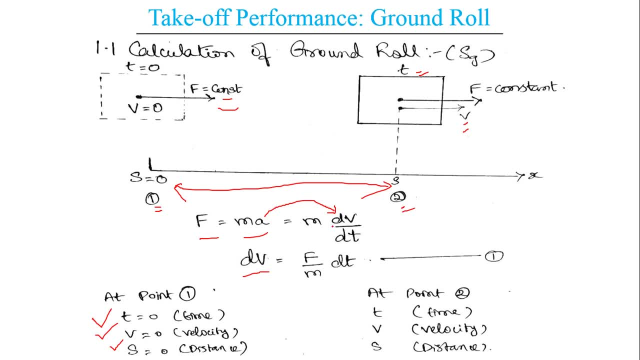 we can obtain the change in velocity dv term by replace the change in velocity dv term by replace the change in velocity dv term by replace the change in velocity terms of the equations. so dv is equal to f. so this ma is simplified. as force f, the m is going to be: 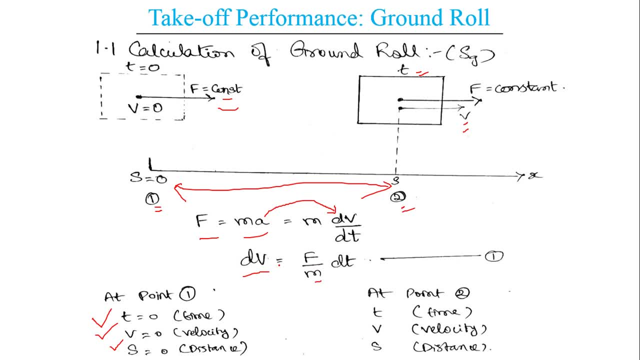 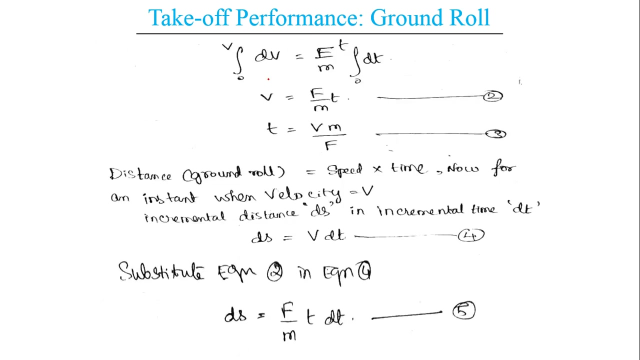 the denominator and dt is going to be multiplied. so change in velocity is f by m times the differential time dt. so here we are getting the terms in differential form, so we need to integrate it in order to obtain the velocity term. so let us integrate it from initial condition. 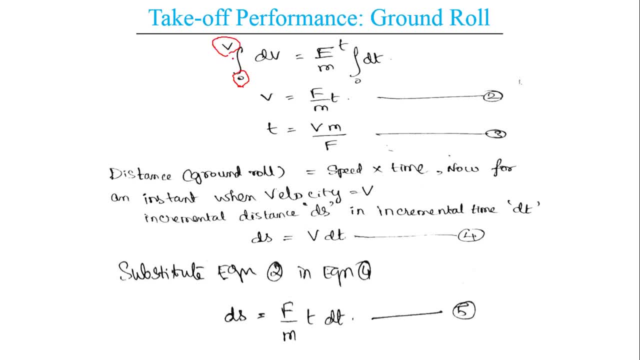 to the final condition. so the velocity is zero at the initial condition and velocity increases to v at the final condition. similarly, the time, so when we integrate it, dv turns to v and fm is constant, force is constant and the mass is also considered as constant. and the time when we integrate dt. 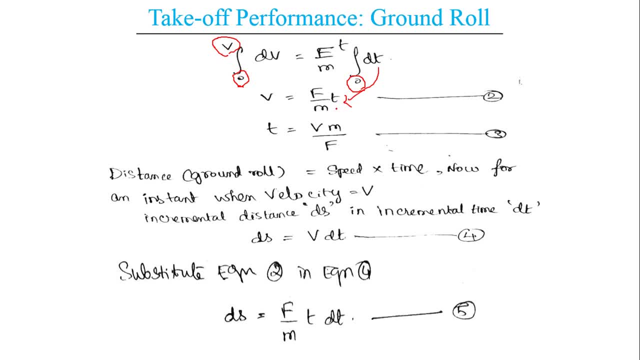 we will obtain t. so here we can rearrange this equation in order to find the time required to achieve this velocity. so if either one of the values are known, we can rearrange the equation and find the other one. vice versa, we, also known as distance, is nothing but speed multiplied by time. 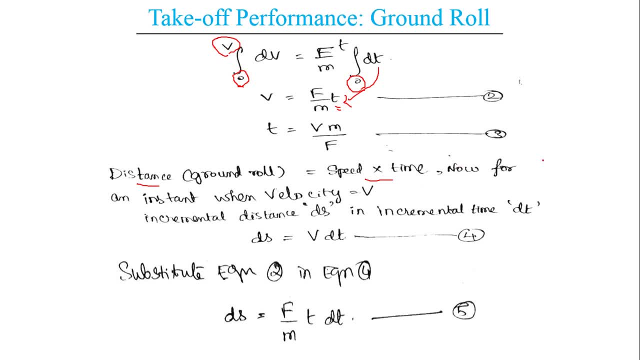 so we know the formula: speed is equal to distance by time. so it is from the same formula: s is equal to distance by time. so s over here is speed and d is distance time. so now, when we need the velocity, now for instantaneous velocity, speed is also the velocity in terms of vector. so when we 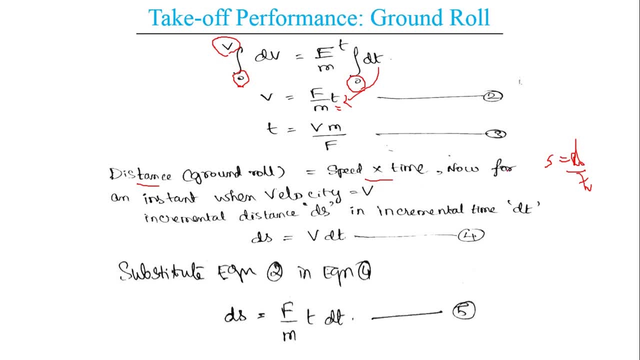 replace the term with v, we can also find the velocity of it. so when we replace this term with dv term and let us consider the velocity is equal to the velocity of the speed is also equal to want Explain v value. okay, now let us come with. the velocity of the speed will be the velocity is attacked. 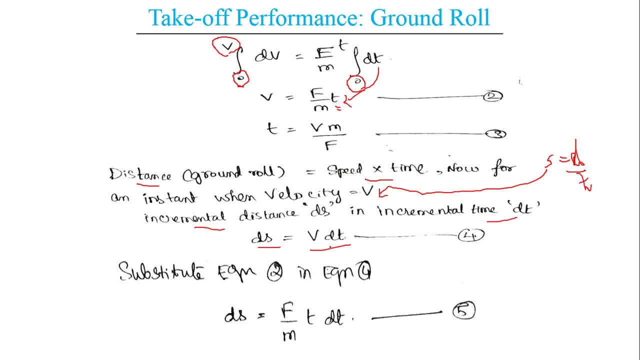 anditsu dau in terms of properties of time, and Ecuadorian and esos and our exact skills. so when we calculate the velocity speed, we can notice that t, which was equal to 4 минут, will need some velocity, and so van der route is required that t should be 0.12 Wars, which is equal. 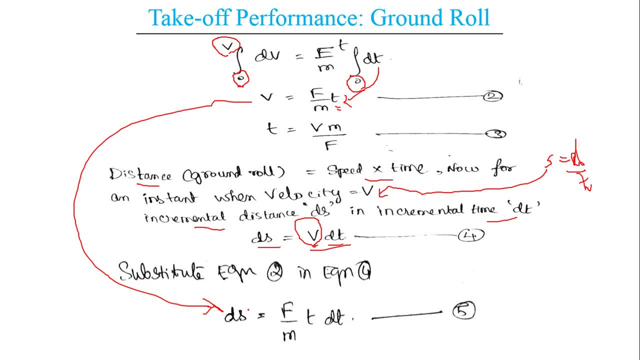 value can be substituted over here. so when we substitute the value of velocity V in equation for round, we can obtain an equation pretty much similar to this. so here we are obtaining the differential or incremental distance with respect to the incremental time. but what we need is the distance, so we can simply integrate. 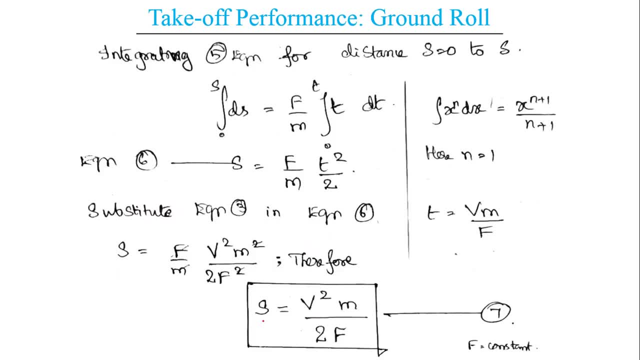 it in order to obtain the distance s. so here, when we integrate that equation, we can see that it is integrated between two values: the initial condition and the final condition. there is 0 to some particular value. so when we integrate ds, we will obtain s, which is the distance. so here, and f by m is constant, force is: 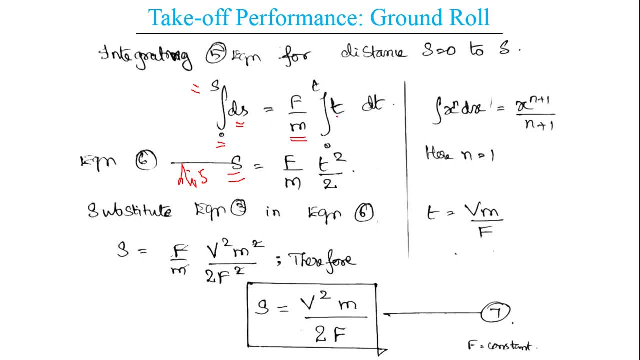 considered to be constant and the mass is also considered to be constant, and as far as the time T is concerned. so here we do not have a single term dt, we have an additional term, t. so when we integrate T, we know the formula: integration of x power n times dx is equal to x power n plus 1 divided by n plus 1, by. 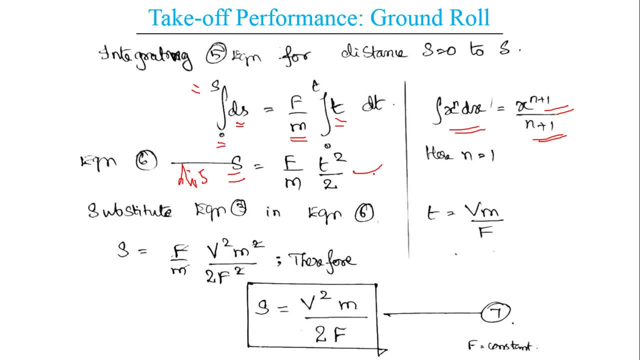 implementing that formula we will be obtaining T square by 2, so we have obtained the relation for distance. so here already to that the time t is also dependent. so we can substitute this value also into the equation 6, which we previously found the value of t in equation 3. so when we 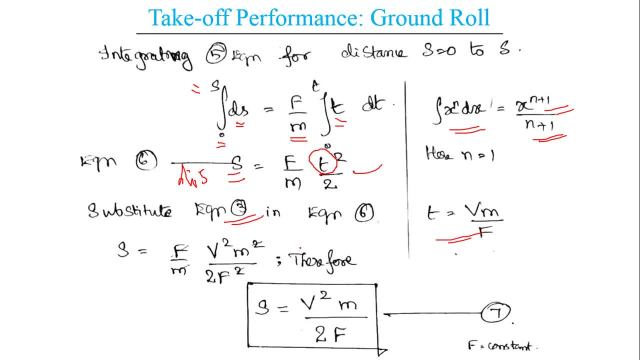 substitute the value of t, that is, b times m divided by f, in the equation 6, we will obtain an equation for the distance. so here, the equation 7 is equation through which we can find the distance. so we know the velocity, and if we know the mass, and if we know the force, we can pretty much find the 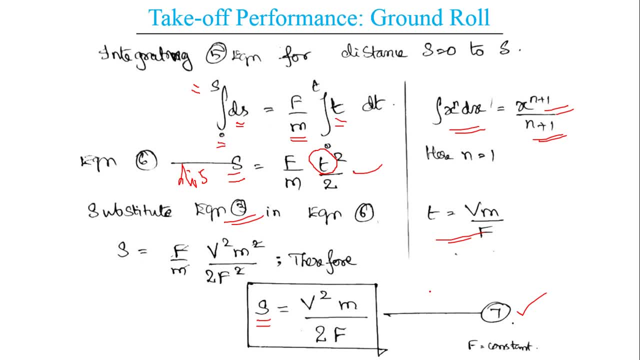 distance. but this is in terms of physics. so how do we translate it to aeronautical terms? so here you can see that it is in common reference as force. so when we translate it into the aeronautical terms, this force is taken in detail or elaborated into the forces acting on an aircraft. that's the 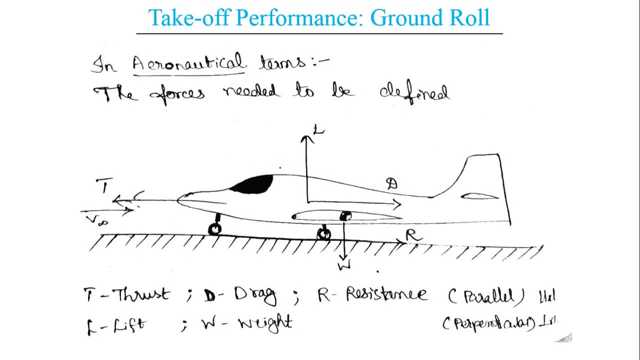 only things which we are going to make. so here we know that during a takeoff, consider that this is the takeoff direction and let us consider the forces on an aircraft. so here we have thrust, lift, drag, weight, and an additional force is added over here: the resistance in general in cruising conditions. we do not 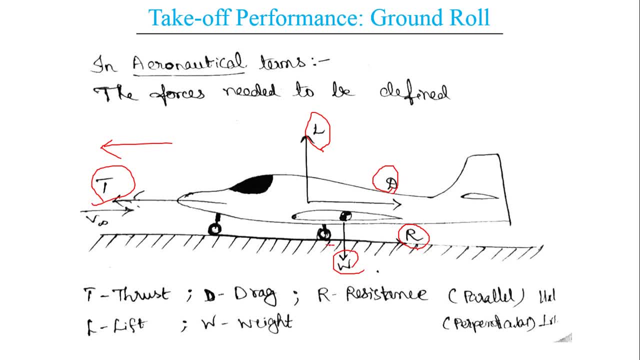 consider resistance, but in case of takeoff there is a contact between the wheel or tire and the ground or the runway, so this causes a pretty much resistance. so this needs to be taken into account for takeoff and landing. so when we consider the forces, let's categorize or group them based on its 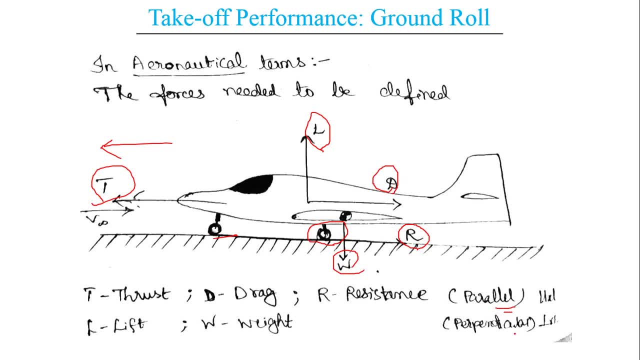 type, whether it is acting in parallel direction or per particular direction. so when you group the parallel forces, there is thrust, so there is also drag and there is resistance. let us consider this is a positive direction, so the forces acting in this direction are considered positive and opposite is a negative. similarly, the forces acting upward is 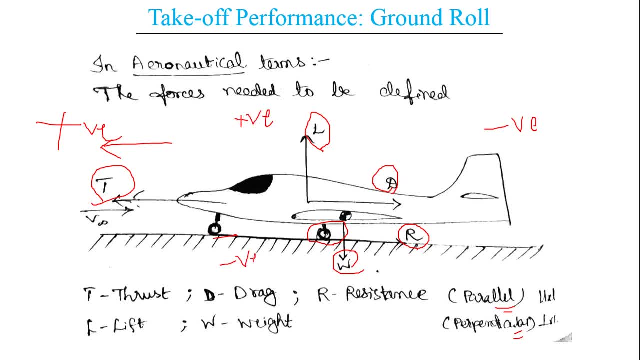 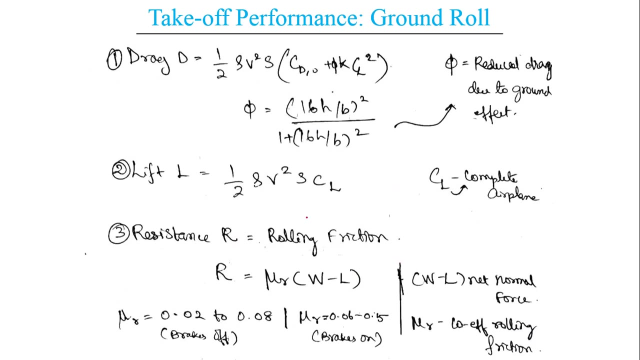 considered positive and downwards is considered negative. so this is a sign convention which we are going to be using. so when we consider about the perpendicular forces, there are pretty much only two forces. it has to be the lift or weight. so we also know that the forces have been already derived from. 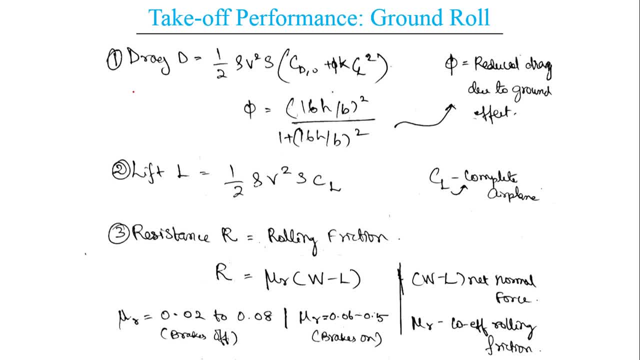 Bernoulli's equation or similar kind of derivations. we can write the formula for these forces. so drag can be written as half rho v square s, c, d and c? d can be defined as c, d naught plus k, c, l square. so this is the drag polar term which we discussed in the previous lecture and further we can see. 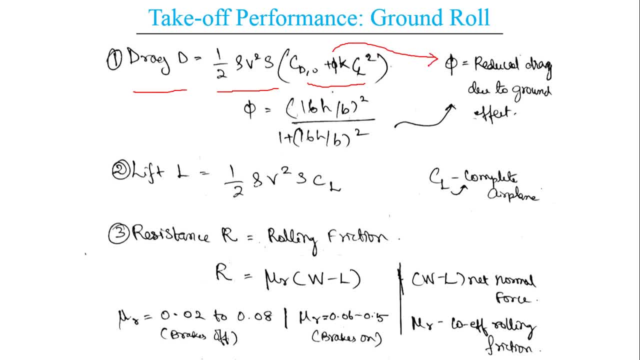 that the effect of ground effect can be added into this equation. as the aircraft is taking off, and as the aircraft is near, or airplane is near, the ground, there is an additional lift produced to the or induced to the aircraft from the ground as the flow gets deflected from the ground. so this: 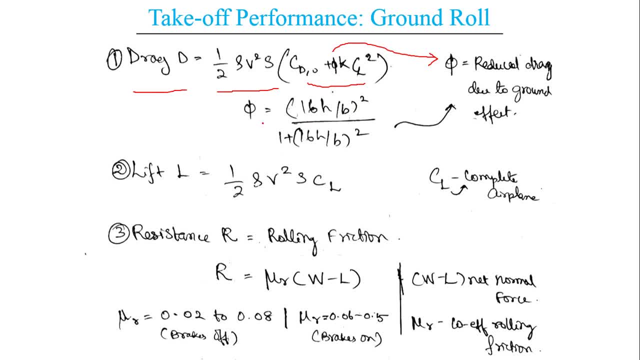 is known as the ground effect. here we can see the formula for phi, and so this was derived. this is an empirical value and it was derived by a scientist, so we can. one thing about this is that we can add as many factors as we can, so this: 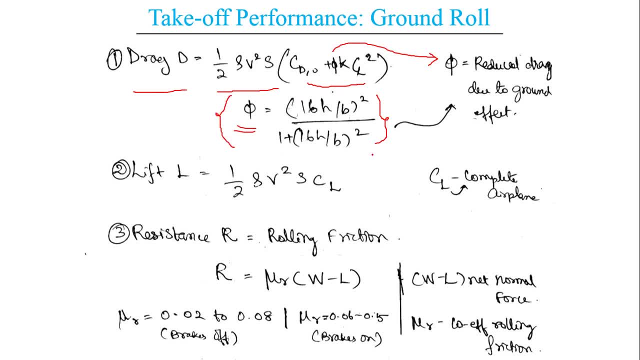 equation gets complicated. our objective is to keep it as simple as possible, so we are neglecting these kind of empirical values. so for accuracy you can still add these. so here we can know that lift is half rho v square s, c l, so c? l. here i would like to mention the l, the capital l term. 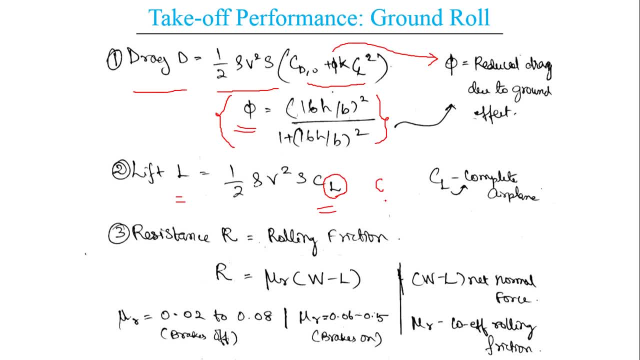 is for complete, complete airplane, and when we see the small l term, it is for a 2d wing, that is, in infinite wing hair foil. so here we did see that we are discussing the parallel forces, so and resistance is also considered. so what is causing the resistance? so resistance is basically. 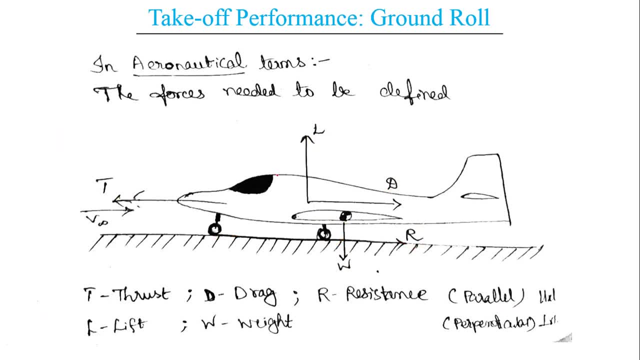 caused by the difference in perpendicular forces. so the forces acting in the perpendicular direction is going to decide the resistance. so it is the difference between the lift. so lift is going to be greater than the way that it Freel, FELting, and also lift minus weight will will be obtaining the net force, net normal force. 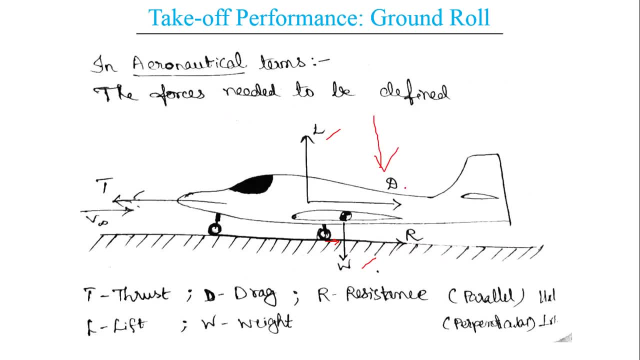 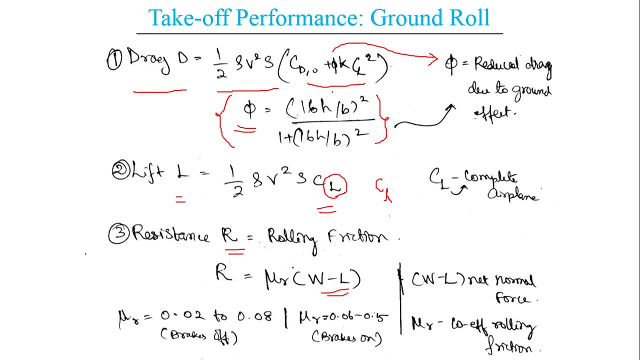 so this is a normal force, normal in this direction. so when we take the difference in the or the net normal force and then we add a factor known as the coefficient of rolling friction, so there is some friction and it depends on the type of the runway. either it is smooth or wet, or either it is a grassland or 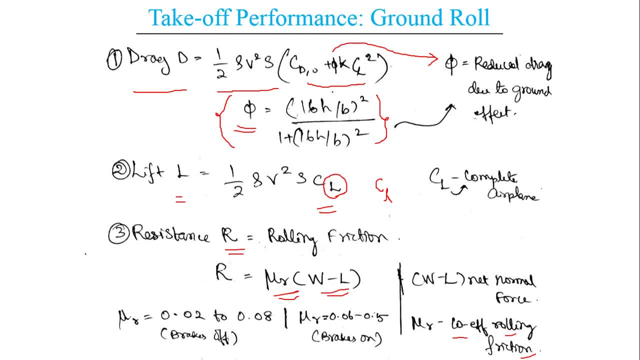 paved runway or there are many kinds of runway, so the value pretty much differs. so here we can see we need to add in coefficient term, then Mu R. so Mu R typically ranges between point zero two to point zero eight four breaks of condition, and when we apply breaks the value increases to point zero six two. 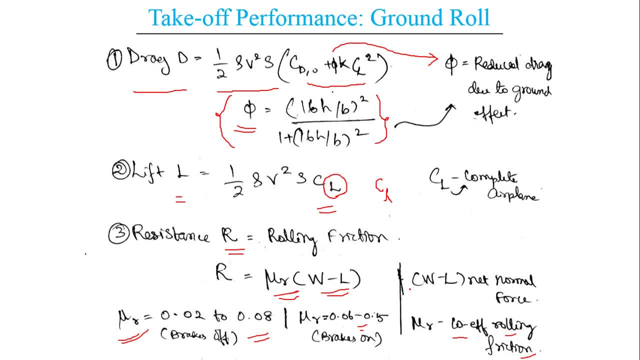 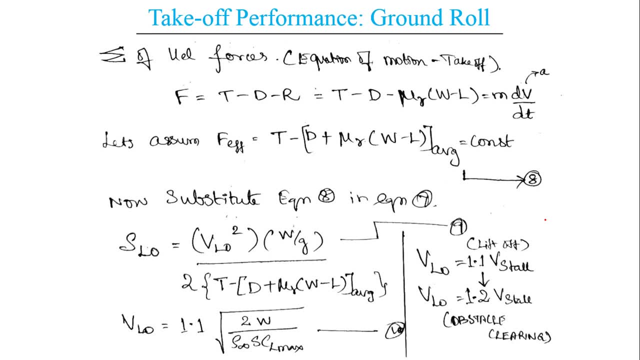 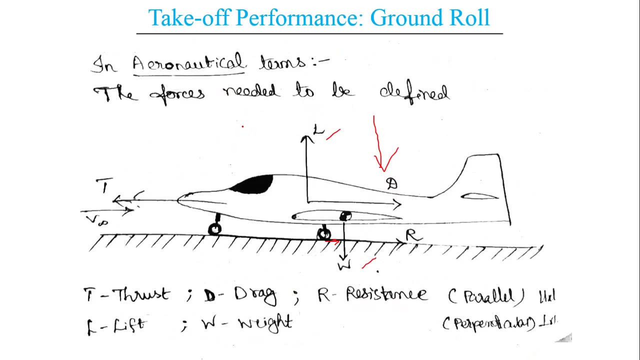 point zero, phi. Okay, now we have derived the, defined the forces, parallel forces. so when we sum all these parallel forces, so force is equal to, thrust is in positive direction, and similarly we have drag and resistance acting in the negative direction. So okay, yeah, thrust is in positive. 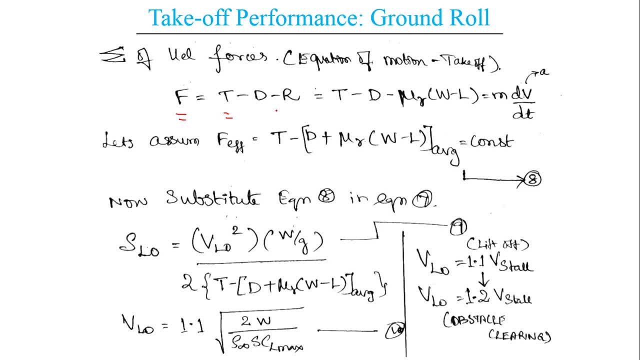 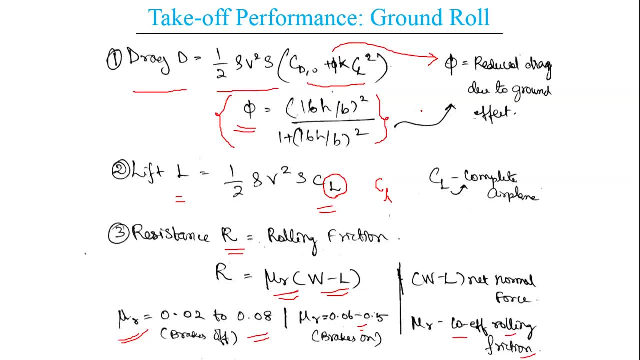 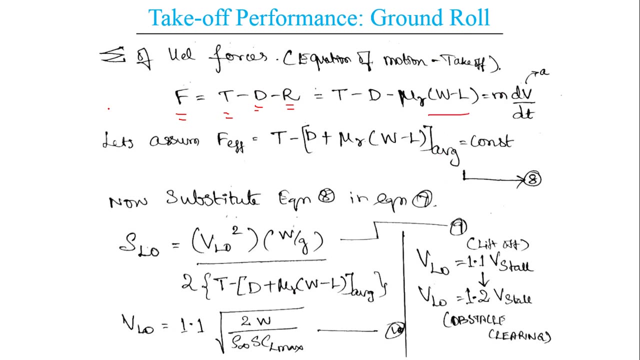 and drag and resistance forces in negative. Let us keep drag as it is and resistance is defined over here from the previous case. so r is equal to mu r times the net normal force, and similarly we know that f? v is equal to m? v from Newton's law. so the acceleration is nothing. 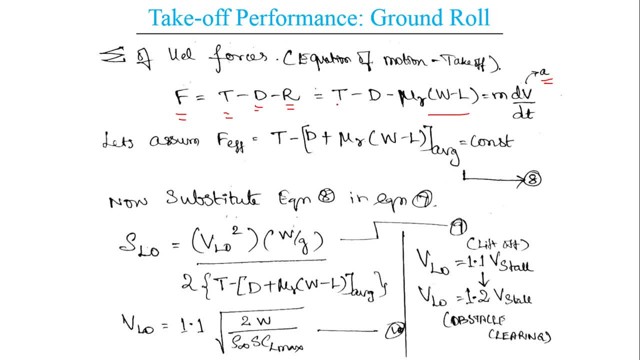 but the change in velocity and change in time by change in time. So here we are equating everything to m is ma. So let us consider this value, so the negative sign is taken common, and let us consider the, this particular value, as an average value, and we need to know that this value is. 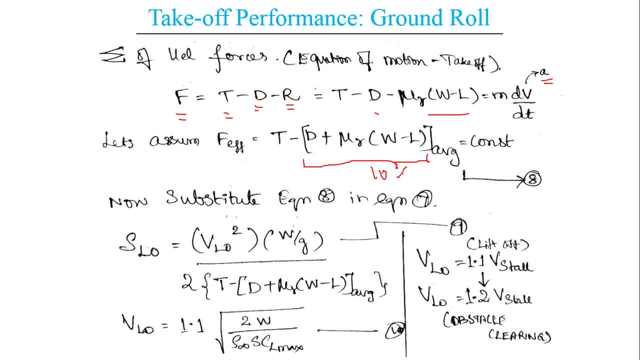 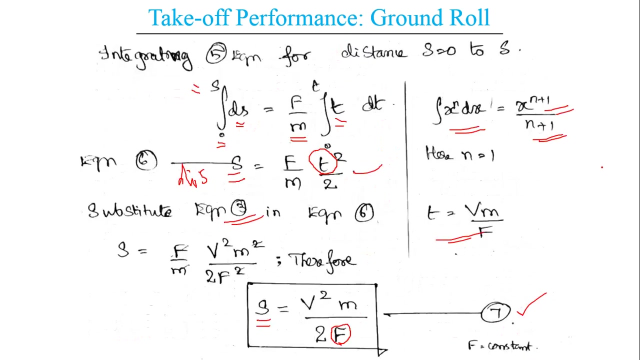 about 10 percent of the thrust. So in many cases these value is also neglected. so let us consider this as constant. So now, when we have obtained the value for f and when we substitute the equation, the value of f in equation seven, So this is the equation seven. so we have defined the value of force in terms of. 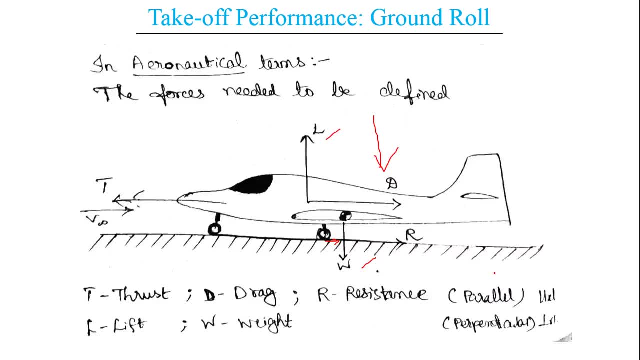 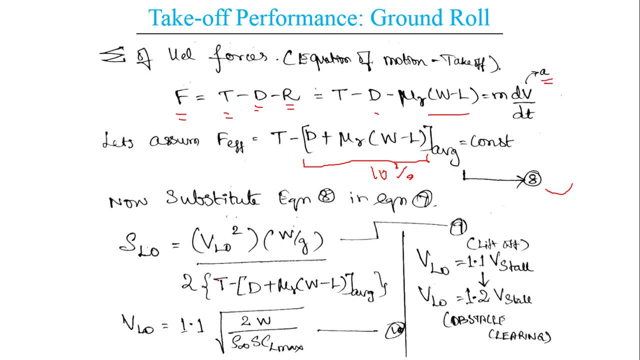 aeronautical terminology, So we have translated it to the aeronautical terms. so v square m by two f, So the f term is replaced with the aeronautical terms of force and m is also written as weight by acceleration due to gravity g. 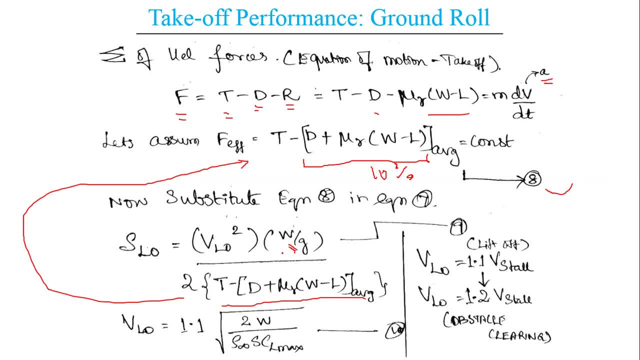 So when we write similar to this and the another thing is that velocity of lift off, as I said in the previous lecture or the previous slides, is 1.1 times the velocity stall, and in stall it is the velocity the lift is equal to the weight. 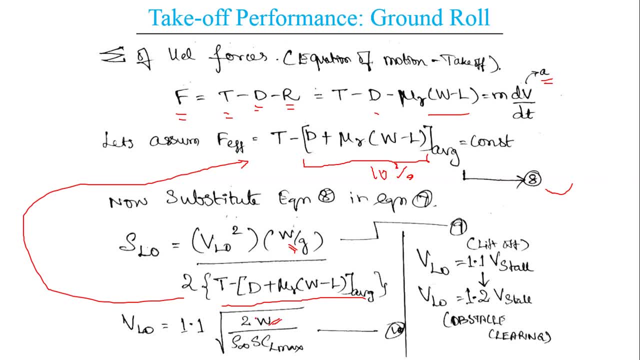 and the velocity can be derived, or the formula for stall can be written as this: and we need to know that velocity of lift off is 1.1 times stall. similarly, the velocity of lift off for airborne distance is 1.2 times velocity of stall. okay, now when we 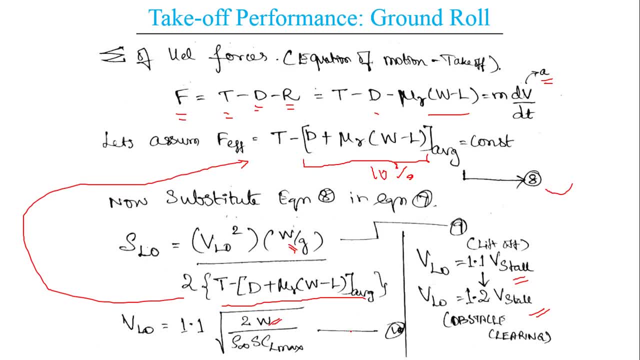 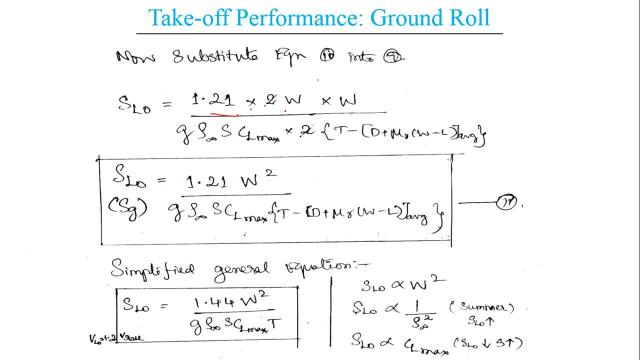 substitute the value of this velocity lift off into the distance formula. we can write the formula as: 1.21 times 2 w times w divided by this, particular terms are included and when we simplify, obtaining an equation which is providing us with the distance required for lift off, and this is: 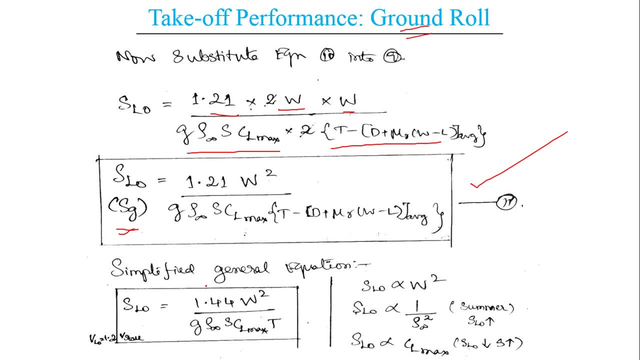 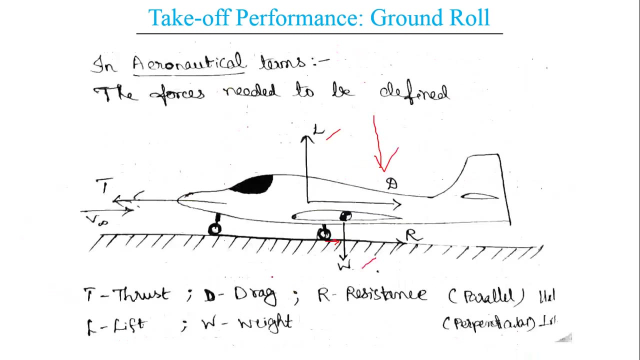 particularly the ground rule. so when we simplify it, instead of taking 1.1 and 1.2 times of velocity stall, we are taking the velocity lift off as 1.2 and we are neglecting the airborne distance. so we are just considering the point at which the aircraft is basically taking off. so when we take 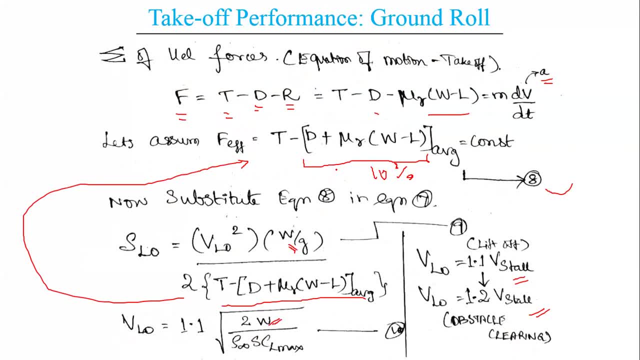 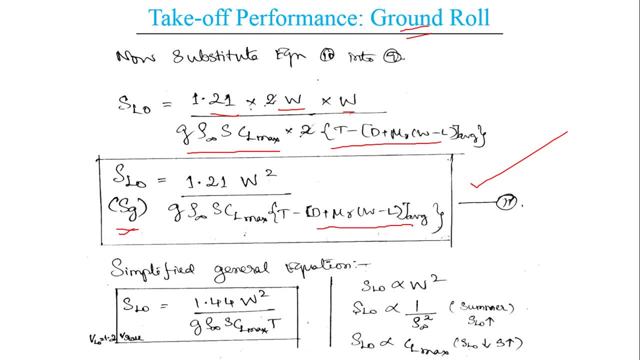 this is indeed incorrect or inaccurate, but for basic conditions we can still consider this, and when we are neglecting the drag and resistance forces, as it is only 10 percent of the thrust, we can pretty much obtain a simplified equation for lift off. so here we can see that the simplified 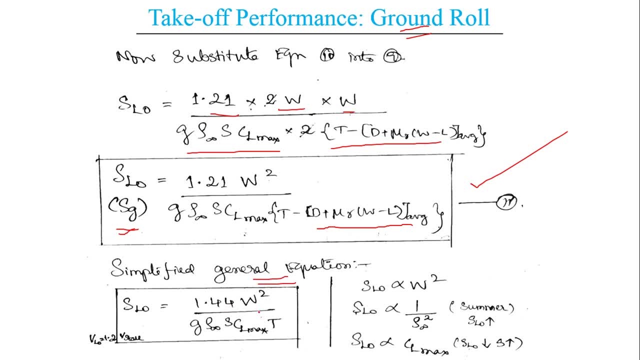 general equation for lift off is 1.44 times the weight square divided by g acceleration due to gravity, and here we see the density, ambient density and the wing surface area in cl. max times thrust for gate perspective. we need to know the relations between these there is. 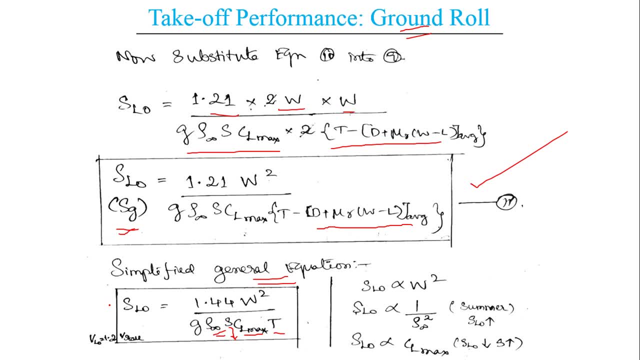 we need to know either the takeoff distance increases or decreases with either of these properties. so we here, we see that the takeoff distance is directly proportional to the square of the weight of the airplane and it is inversely proportional to all these values. so we need to. 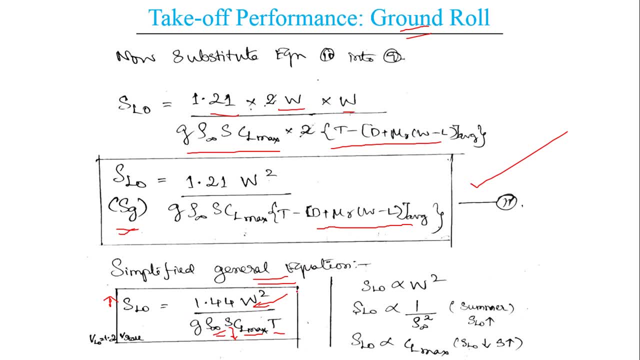 know and this equation can be translated into the physical understanding. so when we see that, there will be questions like if? what if we increase the weight by two times? so when we increase the weight by two times, the takeoff distance or lift off distance is going to increase. 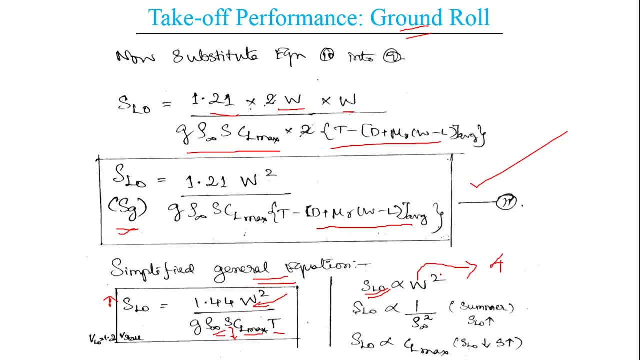 is uh by four times. that is quadrupled, as it is in square terms. similarly, uh, the distance for left off uh is inversely proportional to the density, and when we consider that thrust is directly proportional to the density, it is a square times density. so this is in particularly interest. 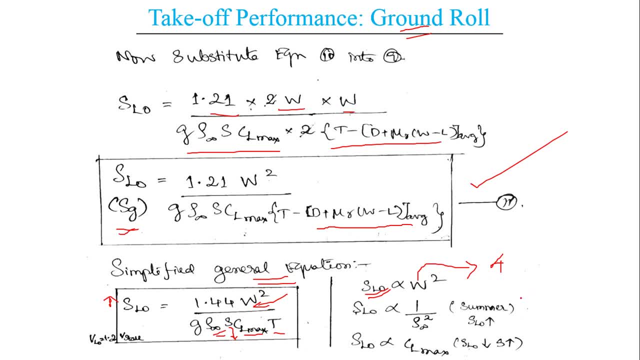 interesting topic, as this is the deciding factor wherein we see that in summers, takeoff distance is increased, that is, we need additional uh runway distance in order to lift off, but in winters, uh, it is uh the reverse case, that is, we can take off from shorter distance, so as the density is low. 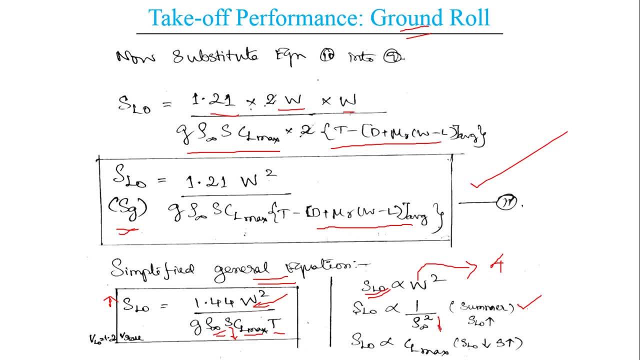 we can see that if density decreases, the takeoff distance increases and if uh, vice versa. so in summer the density decreases due to heating up and the runway distance increases. similarly, we can see that in order to increase uh- here we can see the cl max uh- the lift off distance is uh. inversely, 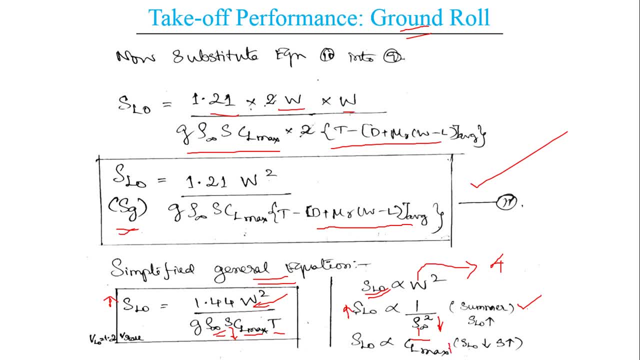 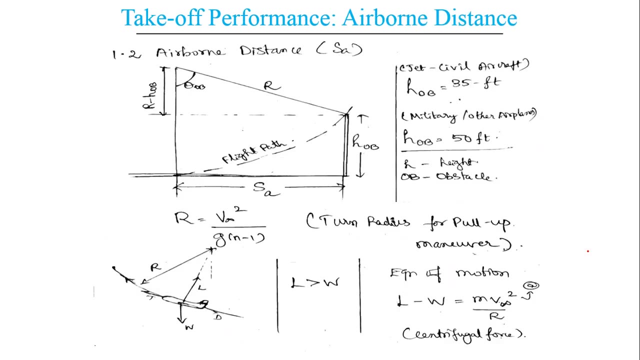 proportional to the cl max. so if we increase the cl max- uh, that is, if we increase the lift, that is, by deploying flare or any other kind of mechanisms, we can decrease the takeoff distance. our prime motive is to decrease the takeoff distance, so we basically do not have infinite distance to take. 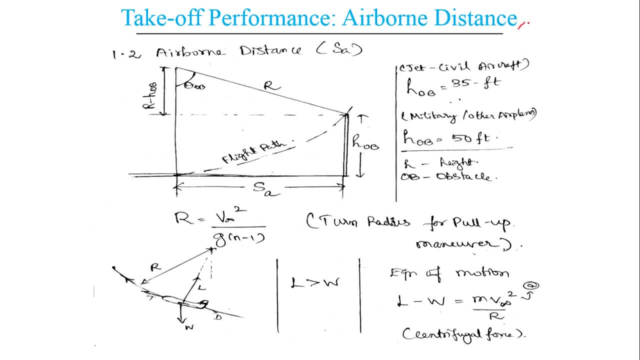 off. now we are dealing with the second portion of the takeoff performance: the airborne distance. so the distance required to clear the obstacle height is known as the airborne distance and, as i said, it varies. the obstacle height varies according to the federal aviation regulation. so it is basically 35 feet. 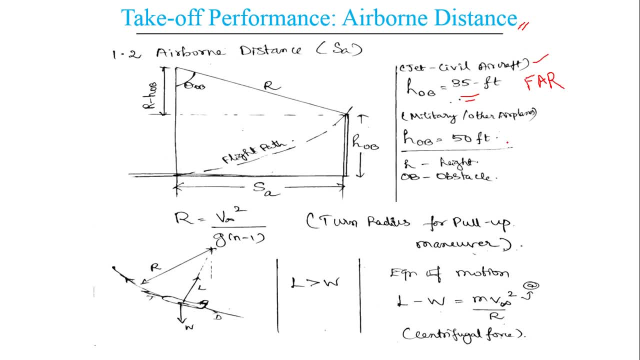 for civilian jet powered aircraft and the obstacle height is 50 feet for military or other airplanes. and here we can pretty much see that the equation can be derived from the trigonometry uh basis. so here we can see we need to find the sa term. so how do we apply trigonometry and find this? now let us consider the. 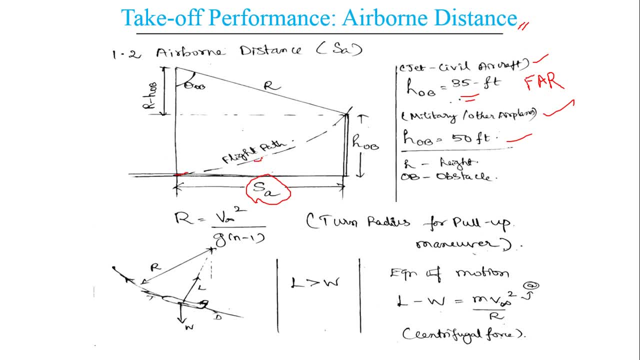 airplane which is taking off is, uh, particularly following some curved portion or a curved line. so when we are, and we know the obstacle height and we you know all of the terms, and by this we know that there is some particular angle it is making with the obstacle height. so 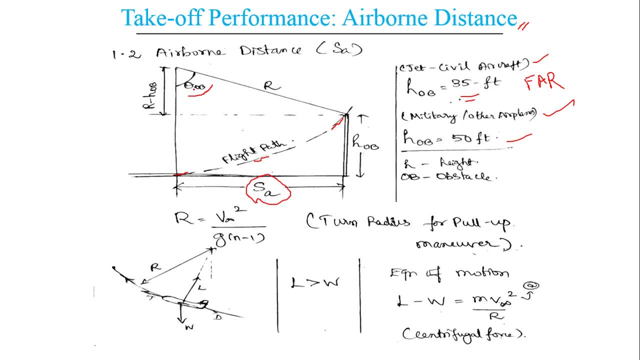 here we call this angle as theta ob, so this is the angle of obstacle height. so here the sa term is same, so this is also and we call it as sa. so in order to find this, we know the theta and for this case we can write: is as sine. theta b is nothing but opposite or cos. theta b can be written as adjacent. 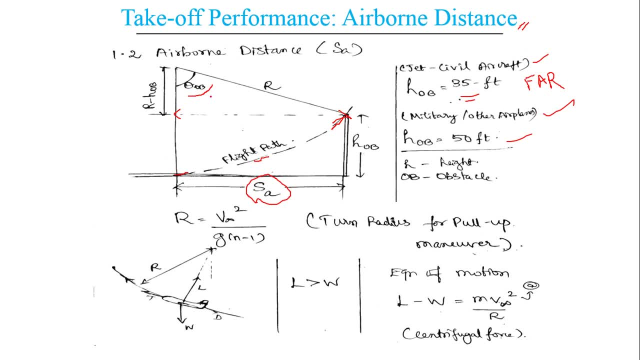 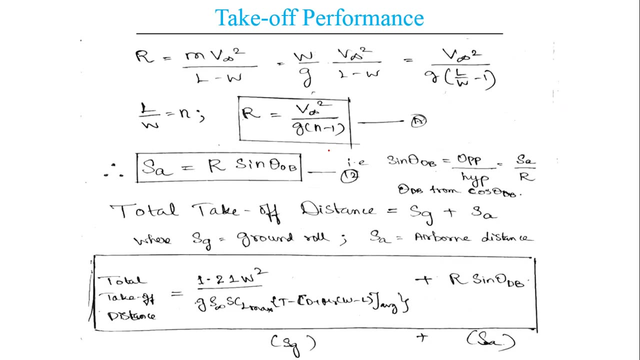 by hypotenuse, we will find about it. so here we are, are concerned with the sa, so distance of airborne, so air bondation, so we need the opposite term, so we are considering the sine theta term. so basically, when we consider the sine theta term, we can. 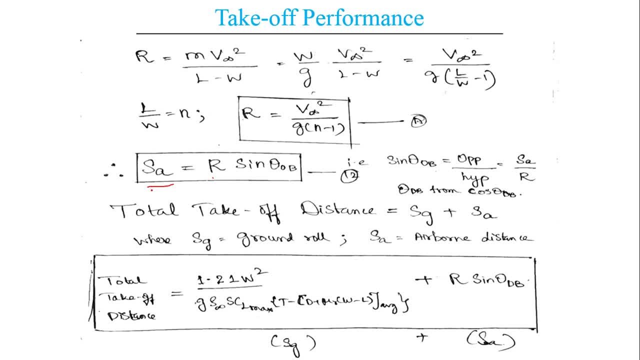 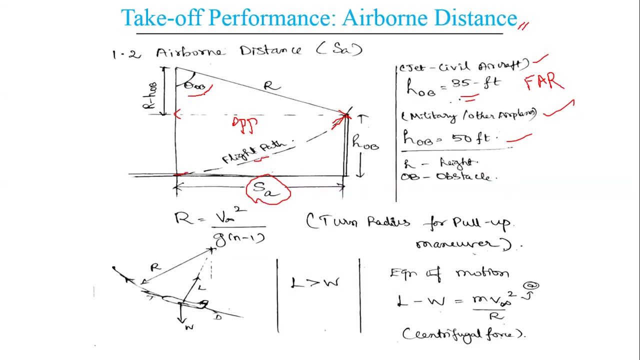 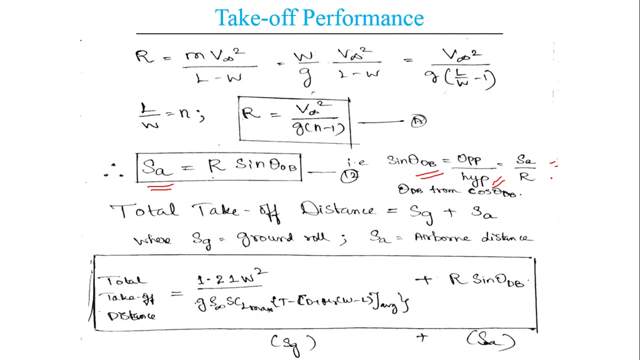 directly. uh write the sa, so airborne distance, as r, which is hypotenuse. so here we can see that sine theta is nothing but opposite by hypotenuse. so opposite that uh, opposite to the theta b. theta ob is sa and hypotenuse is r. so when we take uh, substitute the values, we will obtain like this: 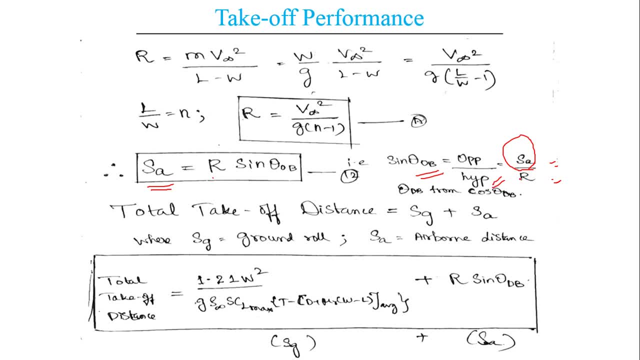 and we need- uh, they say so we are taking the r to the lhs term, so we will pretty much obtain the airborne distance, as sa is equal to r sine theta zero ob, that is the obstacle height. so here we need to know what is r. let us assume that we know the theta b by substituting some kind. 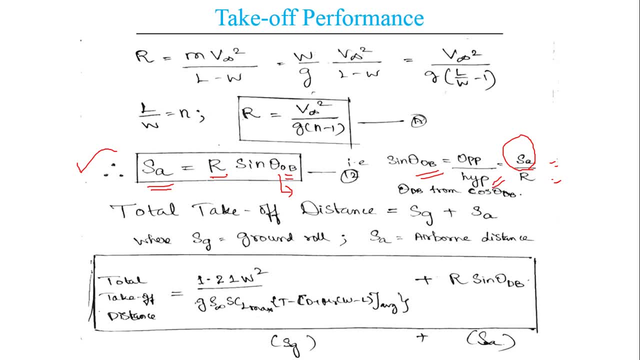 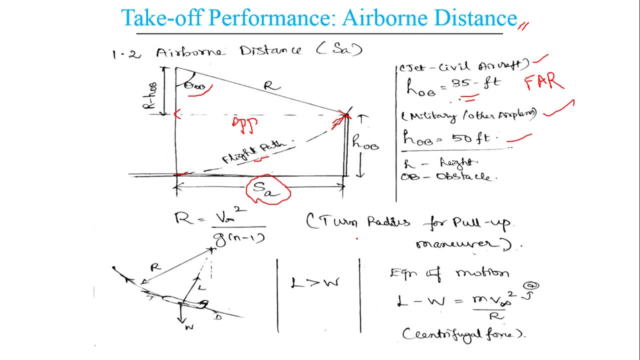 of trigonometry equation. so what is r, r is nothing but the turn radius. so this turn radius is basically obtained from the pull-up manual. so we need to know what is pull-up manual and we need to know how to derive it in order to know about this. so consider that an airplane is, uh, in a pull-up manual, so the lift. 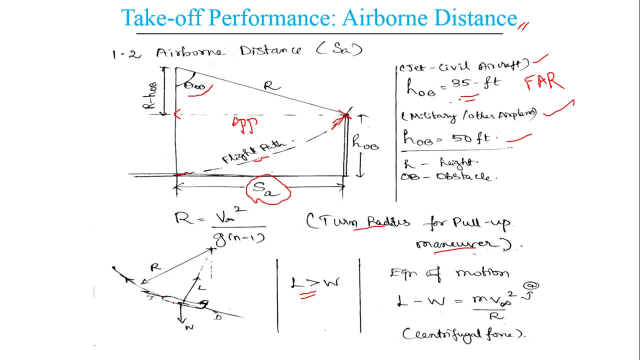 is basically going to be greater than the weight and it is going to be following some particular curved path. so let us take the net normal forces. lift minus weight is equal to f, is equal to m a. so this is the net normal force and this is the mass times. this term is the acceleration. 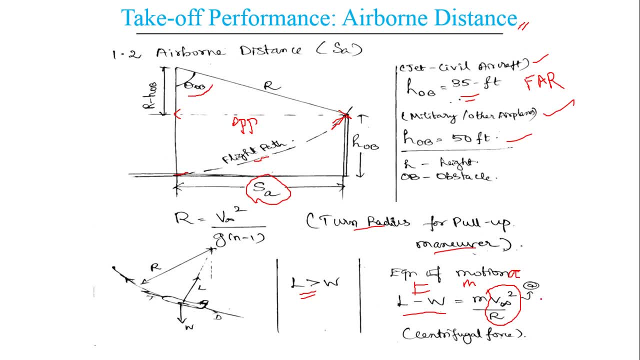 so here we can see, acceleration is not dv by dt, instead it is v square by r. so this is uh, basically uh for the acceleration which is caused when an object follows a curved path, and uh, this is a special topic and the of physics, and uh, it is uh. 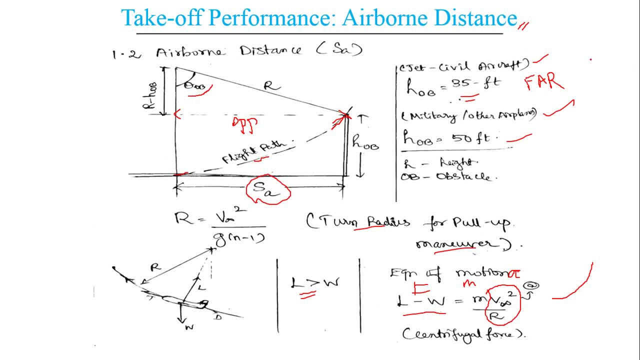 very well explained by professor man matt and lexon. so link to the session will be provided on the right top corner as youtube cards. you can refer that or you can also refer your school books of physics. so this mv square by r is nothing but the centrifugal force. 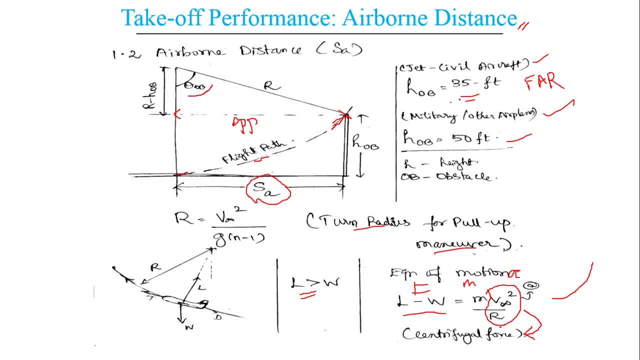 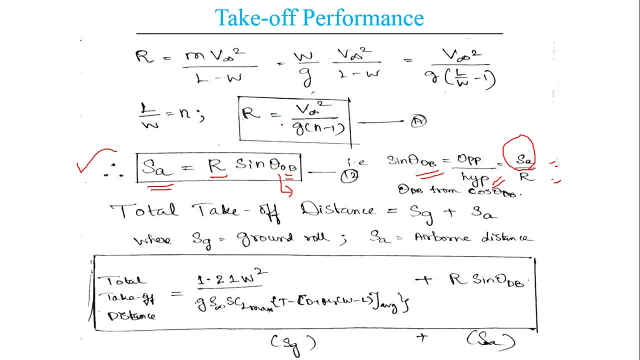 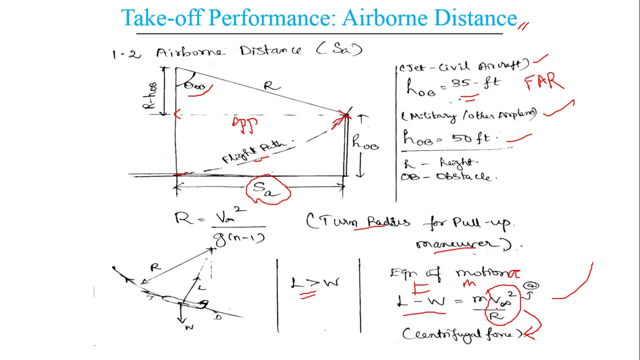 okay. or when you search for this mv square by r, you can search by the term centrifugal force. so here the r can pretty much be derived from this particular equation. so here we have: l minus w is equal to m v square by r, the centrifugal force. so when we replace the terms, or just 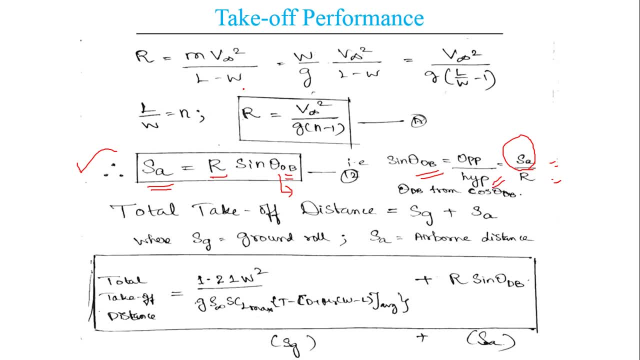 take the r to the lhs and we bring down the l minus w term to the rhs, we obtain a similar kind of equation and the mass can be written as weight divided by gravity. and in that case we can write so: l minus w. we have c w in both the numerator and denominator, so we are dividing. 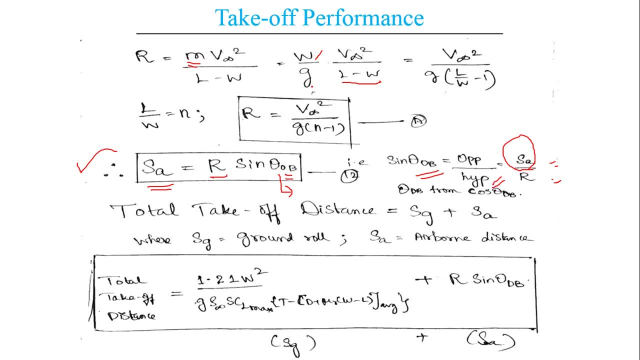 the numerator and denominator by w. so here we can try: uh see that this gets cancelled out, and here this also gets cancelled out. that is one, and we have been remaining with the term l by w. this is nothing but the load factor n. so this is a load factor n when we replace this with the load factor. 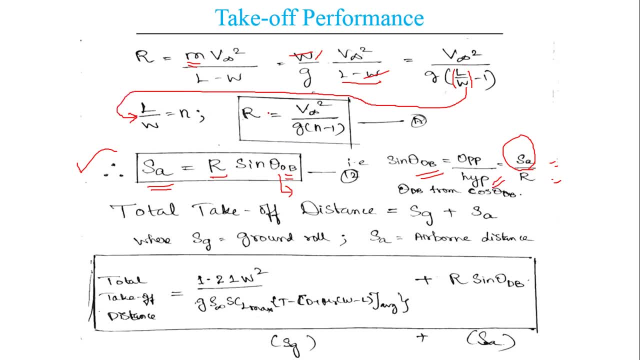 n. we can write the turn radius r as v infinity, squared by g times n minus 1. so this is basic equation for pull up maneuver and for pull down maneuver. this is just replaced with a positive sign as lift and weight operates in the same direction. so as for now, we are concerned with 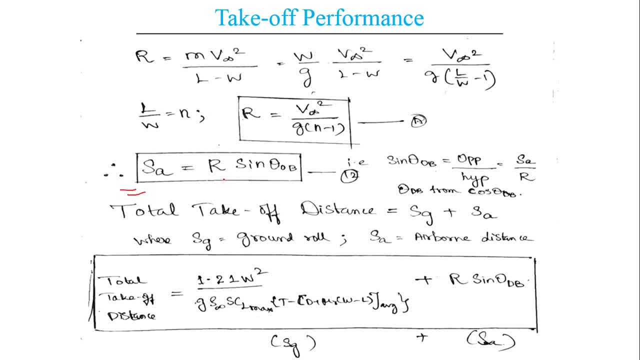 the approach distance, airborne distance, sa, so it is nothing but r times sine theta b. now when we combine the ground roll distances, g value and sa airborne distance value, so here we can obtain the total takeoff distance. so this is going to be, uh, the equation when we obtain 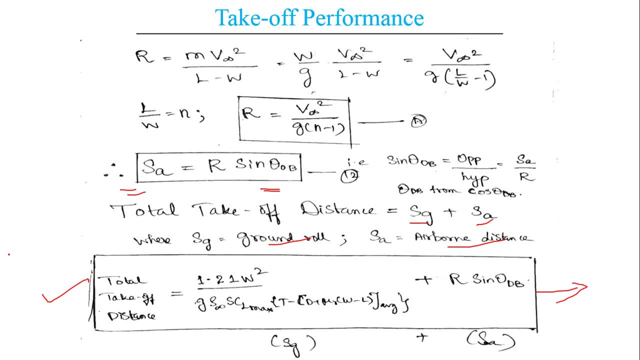 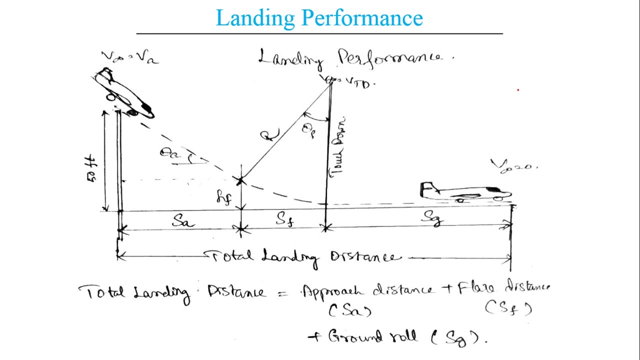 for total takeoff distance. so the total takeoff distance s can be found out if we know the all these properties. so this is theta over here. so this is uh, pretty much what is takeoff performance and how we will get in get into the landing performance. consider that an aircraft which is at some 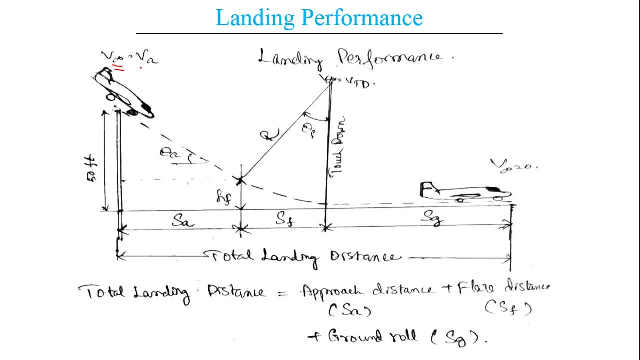 particular velocity and we consider it is approaching the runway. so the velocity is considered as approach velocity and the when it approaches the runway it is going to be approaching from a particular angle. so this is approach angle. and when we are concerned with landing performance, basically the landing performance. 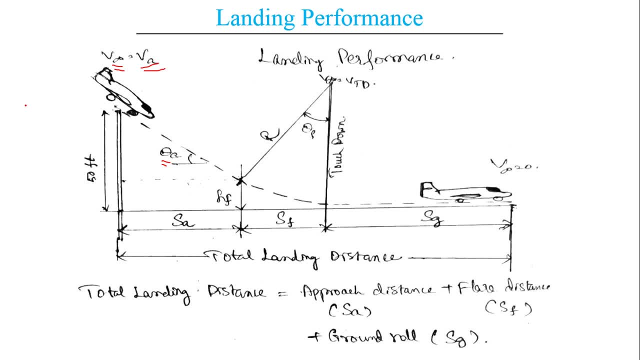 will be taken into three segments. so similarly, as per the fair federal aviation regulations- uh rule our law- we can see that it also needs to clear an obstacle height of 50 feet in order to consider it as landing. so when an aircraft has cleared 50 feet obstacle height, it is considered to be landing, and then further we will. 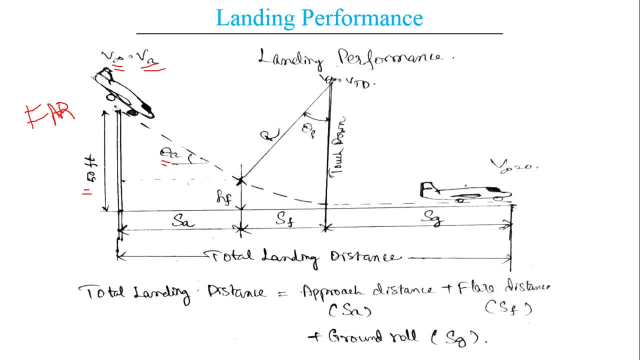 divide the segments from the approach to the velocity zero as three segments. so the total landing distance can be divided into three segments. first is the approach distance, so, as we are concerned with the distance, so here approach distance so, and the next is the flare distance and the third one is the ground. 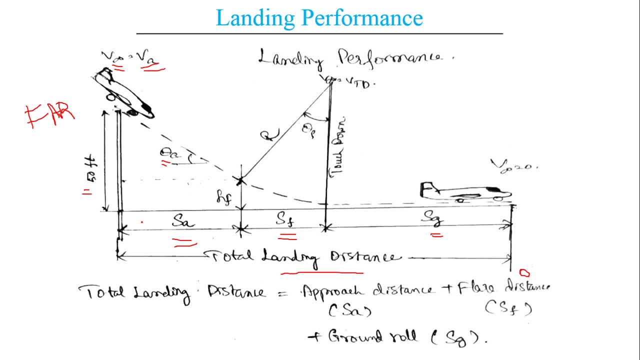 roll distance: approach distance is the distance covered by the airplane during its approach and the flight distance is a distance covered when it is in transition from the approach, kind of so here the aircraft is in inclined orientation and during touchdown the aircraft is going to be in horizontal orientation. so this transition that is covered during this transition is known as. 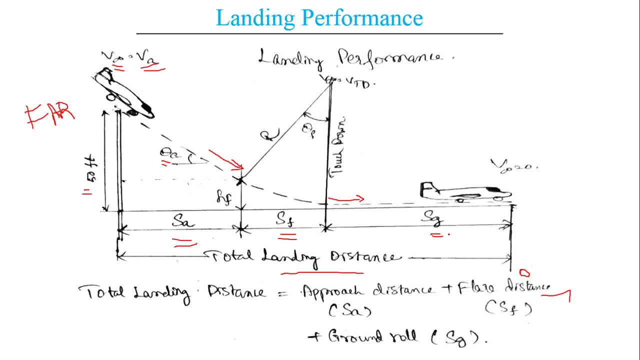 the player distance. this is the SF, and the S G is similar to the the ground roll of takeoff. So here the SD is nothing but the distance covered by the aircraft or the airplane from touchdown to the distance at which it is brought to rest. So this is. 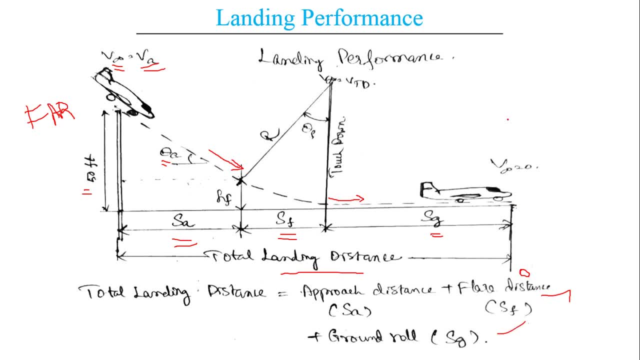 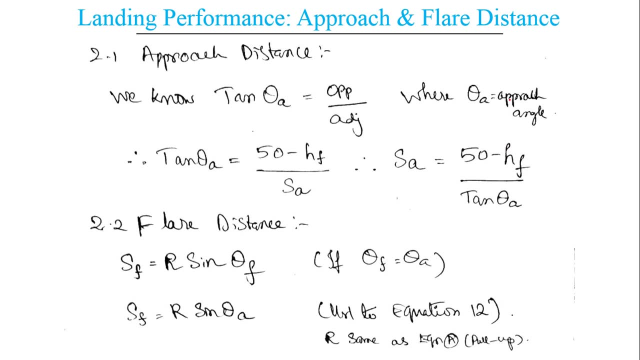 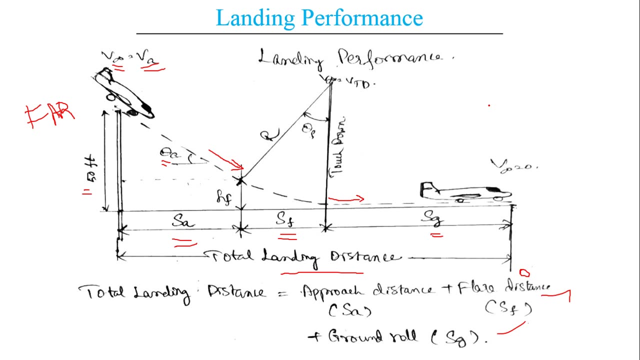 the ground roll distance and we need to note that landing performance is the reverse of takeoff performance. So the landing performance values can be pretty much obtained easily or simply from the trigonometry equation or laws. So approach distance, as we see this forms a triangle over here till the flare height. we consider that up to this height. 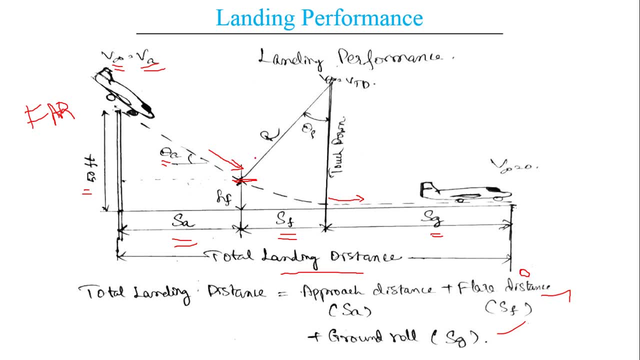 the aircraft is carrying out the same inclined motion. So by using the laws of trigonometry we can pretty much find the SA. So SA over here is in adjacent portion. So we will be obtaining it from the trigonometry equation. So we can pretty much find the SA over here. 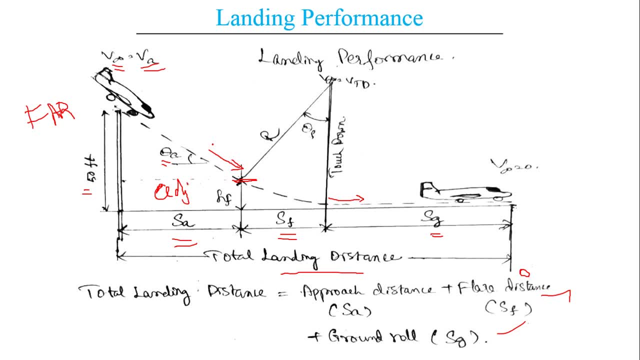 from cos theta. So here, when we need to obtain this, we can obtain it by tan theta, because we don't know what is the value of the hypotenuse region. So here we know the value of opposite region. This is 50 feet and we are considering from hf the flare height, So 15 feet minus. 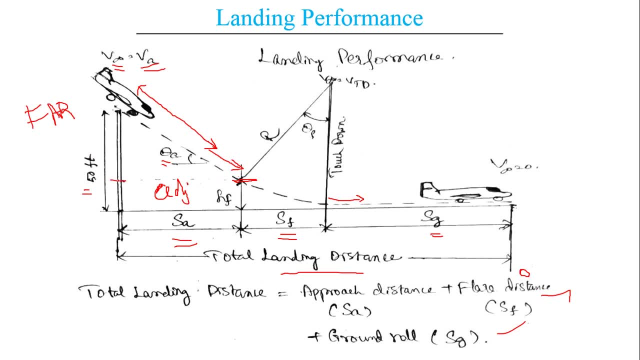 hf will be the height of this particular portion. So when we consider this, we can obtain it by tan theta, because we don't know what is the value of the hypotenuse region. So if we consider that we can obtain the value of SA from the tan, So that is the tan law, So tan theta A is nothing but opposite by adjacent. 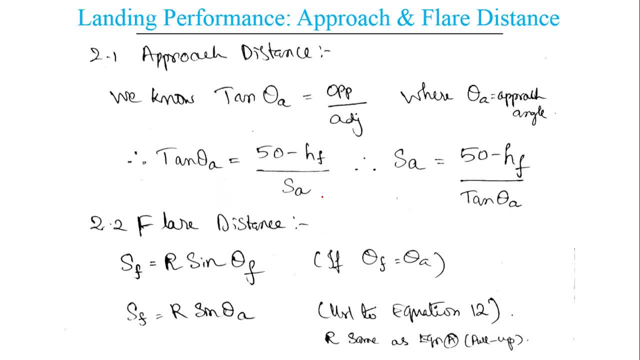 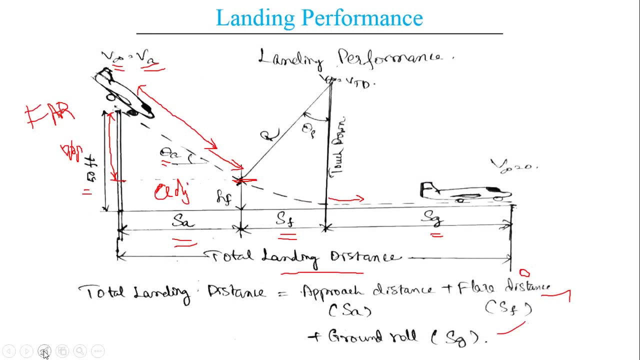 So here we know that opposite value is 50 minus hf and adjacent value is SA. So for finding out SA, we are rearranging the equation, So SA is nothing but 50 minus hf by tan theta A. So the next portion is the flare distance. We need to find the flare distance, So this: 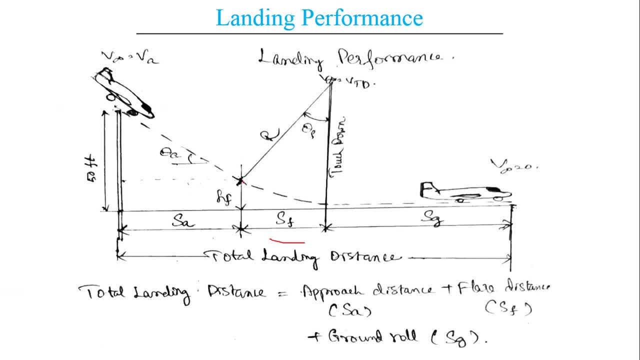 is the flare distance. So flare distance is similar to the pull up maneuver. Here we are not pulling down, So in pulling down maneuver the path will be similar to this and in pull up. So this is the pull down maneuver and pull up maneuver the path is going to be similar. 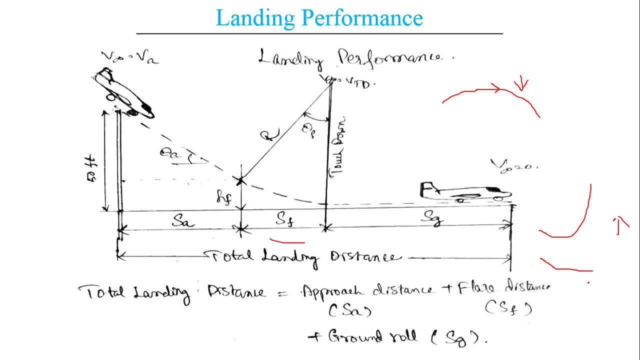 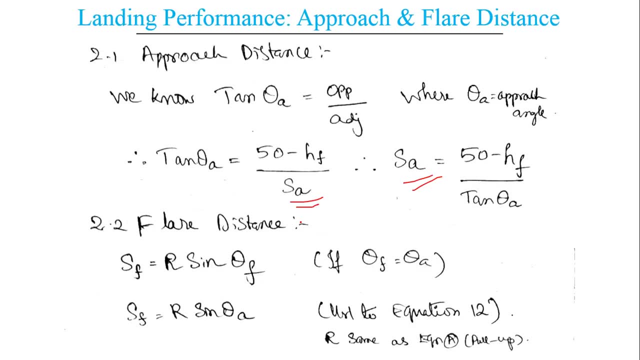 to this. So here we can see that this is the pull up maneuver. So when we consider this, it is same as the previous case for takeoff. So it is the flare distance when applying the pull up maneuver case is nothing but r times by. 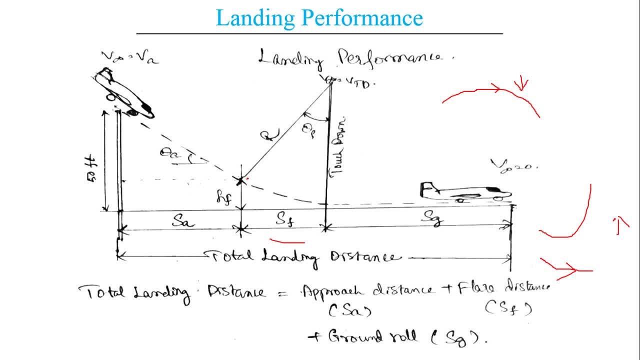 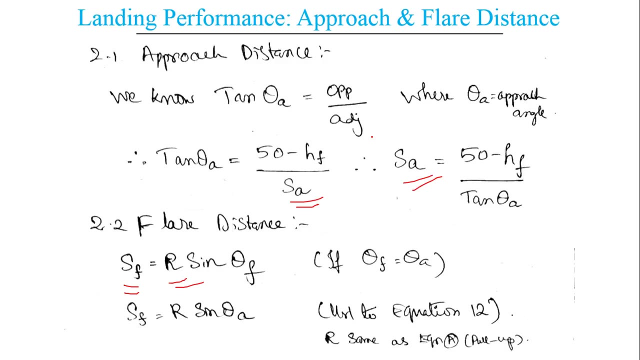 applying the trigonometry law. So it is nothing. but here we are concerned with the opposite side, Sf. So pull up maneuver Sf. Sf can be obtained from the sine theta law, similar to that of takeoff performance, So Sf is r times. 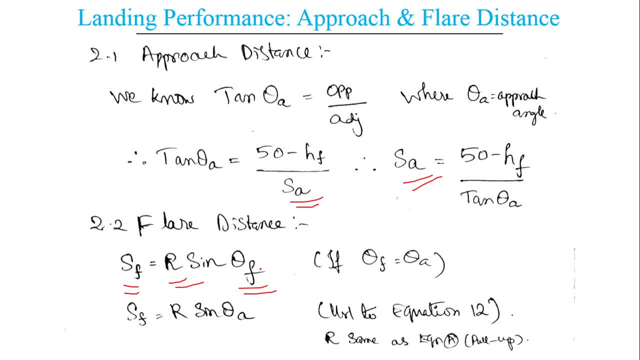 theta f. So this is the angle of flare. So, similarly, this is as I said, that is similar- from the equation derived in takeoff performance and r value can be obtained. the turn radius can be obtained from the pull up maneuvers equation. So equation 12.. So this is. 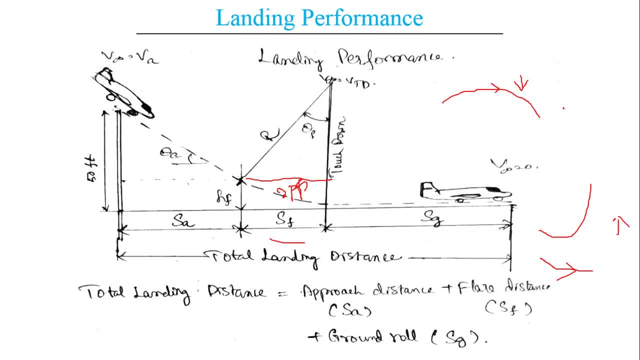 the equation for obtaining the turn radius. It is same Need to remember that here pull up is being taken into account, and it is being pulled down because the value changes. Now, when we are concerned with the third portion of the landing, the ground roll, So ground. 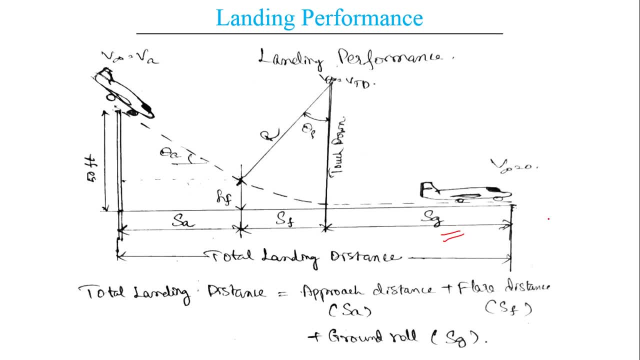 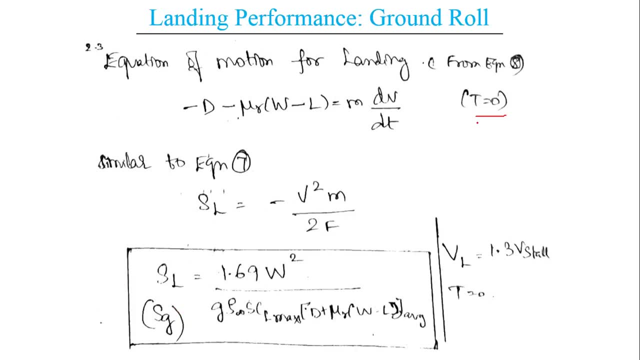 roll is pretty much as same as the takeoff performance ground roll, but it is in the reverse direction. so thrust is taken to be zero because once the aircraft touches down, the aircraft decelerates to zero, the engines are turned off or in some cases, reverse thrusters are used. 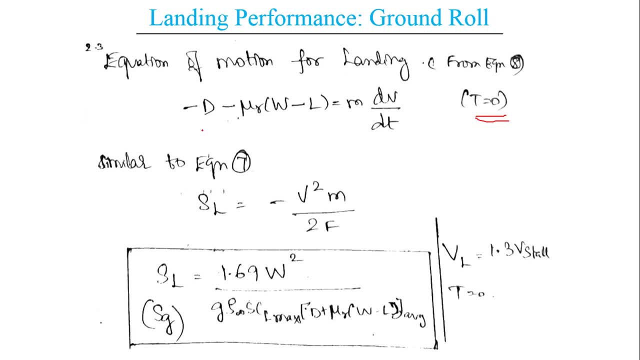 so in that case the equation differs. so when we are considering this similar to the takeoff performance and in reverse direction, because in takeoff the aircraft is in this direction and it is taking off for, so we are accelerating, so landing is pretty much reverse of it- 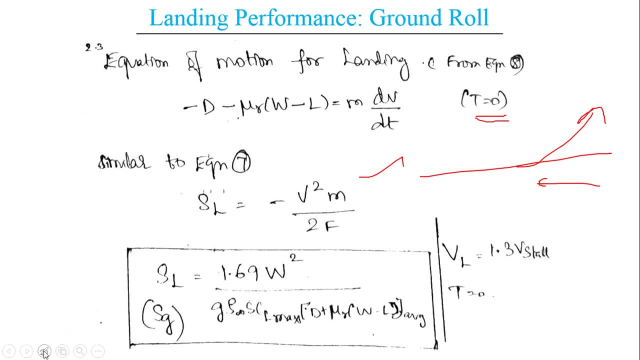 so we are decelerating to some particular value. okay, so we are basically taking uh the equation seven so, which was derived from the laws of physics. i in particular lead the reverse direction. okay, but uh, one interesting point over here is that the force which is uh mentioned over here, so 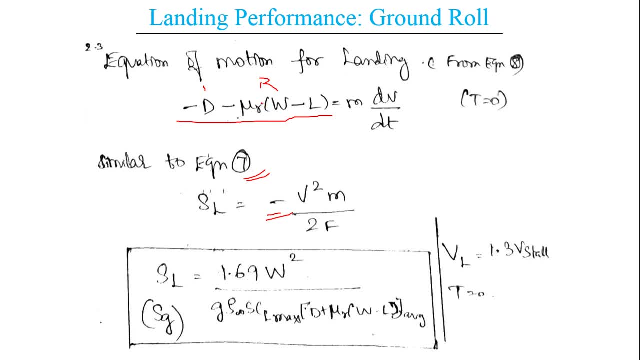 this is a drag term and this is the resistance term. all in negative value and the thrust is taken: zero. so this negative value of this four and the negative value of this distance calculated, the derivation gets cancelled out. so when we take in common, we can cancel out this. so that is why we are writing. 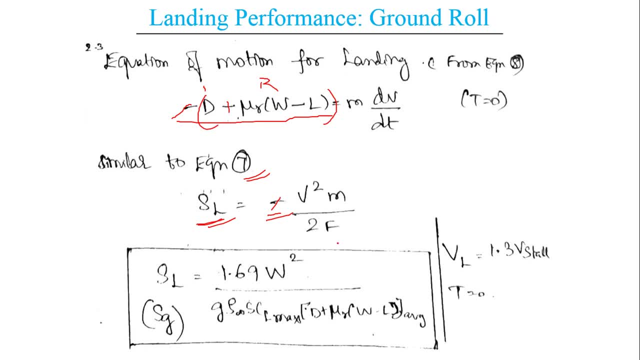 uh, similarly uh. when we uh substitute the value of force over here, we can see that that plus mu r times w minus l and the average value of it can be taken. so this is same. so here this is similar to that of takeoff, but one particular thing is to be noted over here. uh, that is the velocity of. 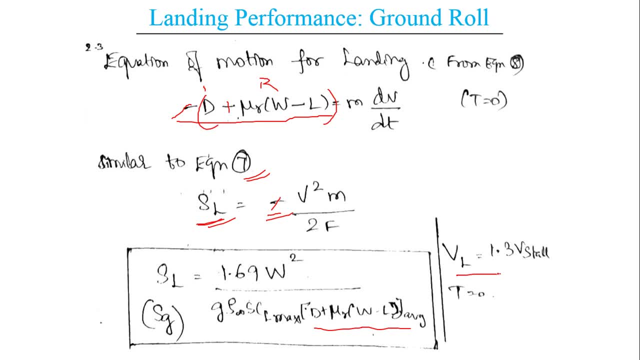 uh landing uh is 1.3 times the velocity of stall. so that is v? l is taken as 1.3 times the stall velocity. yeah, so when we square this 1.3, we'll obtain 1.69. so this is the equation for. 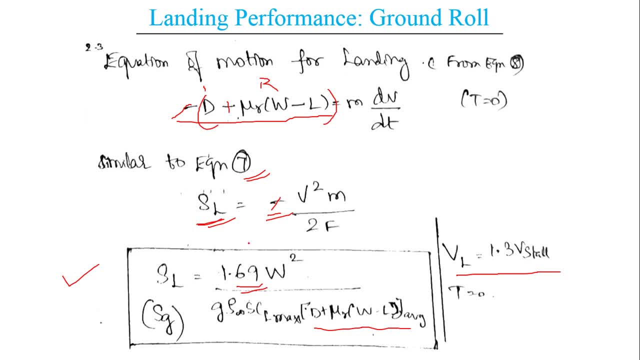 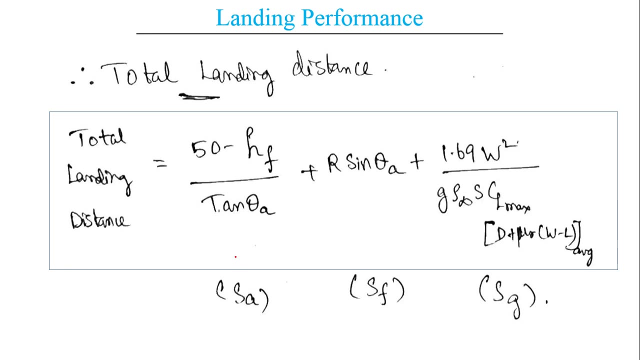 landing ground roll distance. and when we take in common, we can neglect this term- and this particular equation is taken without considering the approach and flat distance. so here, when we sum all these value, the value of approach distance, the value of distance and the value of ground roll distance calculated, we obtain the total landing distance. 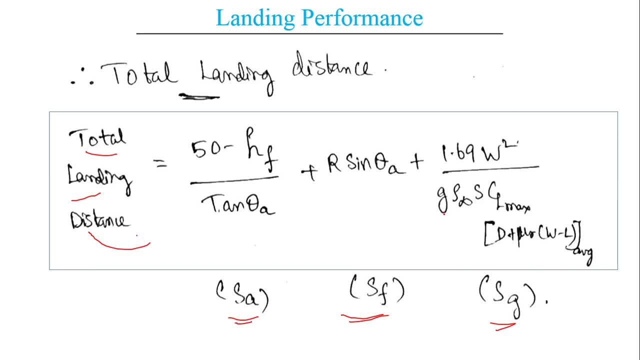 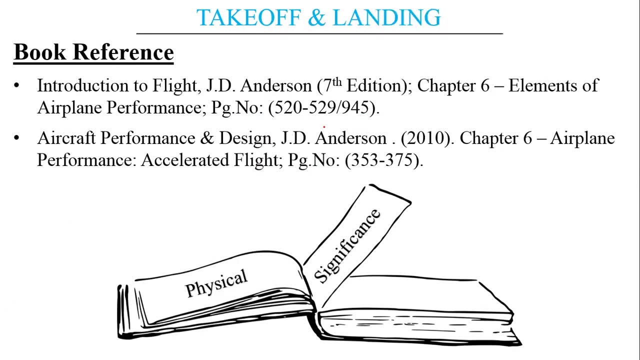 so when we know all these properties or values, we can obtain the flat distance in meters of it. now this is a summarized portion of what is totally regarding the takeoff and landing. for a detailed perspective we can still refer the books. you can obtain the common perspective from introduction to flight by JD Anderson in the 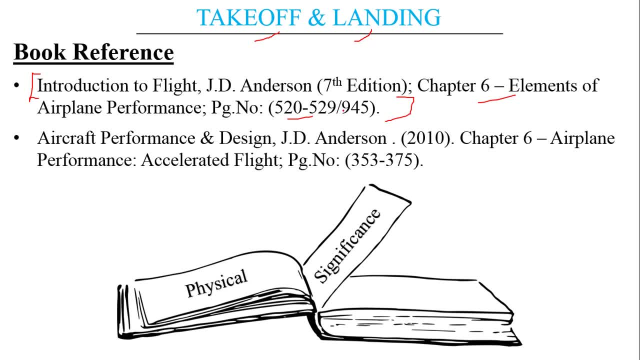 chapter 6, page number 520 to 529, and for detailed perspective there are further more factors added. you can refer the aircraft performance and design by JD Anderson and the chapter 6 of it, airplane performance- accelerated flight. you can read in detail about the takeoff and: 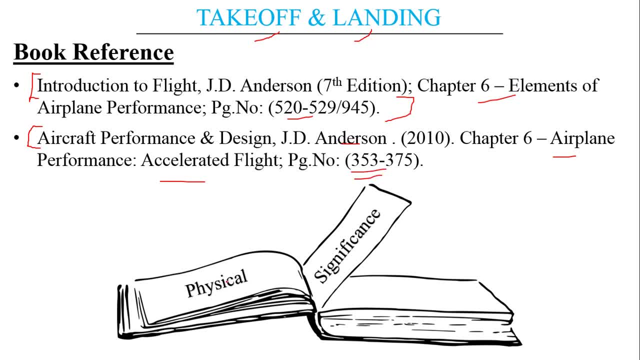 landing. so now, this is a main portion where. where are we using it? why are we calculating this take off and landing distance? what is a physically physical significance of it? this is important because we see there are many aircraft taking off and landing and we can see that few are getting crashed, similar to the recent incident of call ecord er in diya flight. 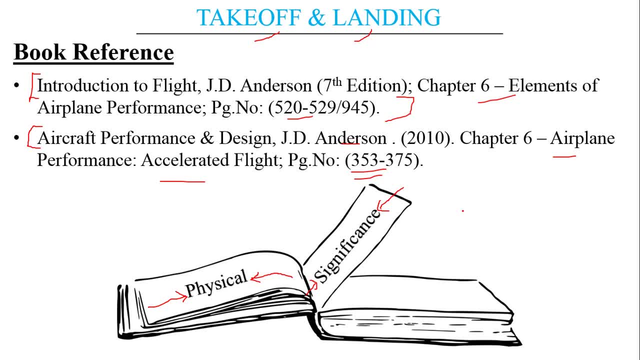 where you can see they are flying after much larger distance. so it indicates that they, which got overrun on the runway- because I am just speculating- consider this as runway. the runway was short as it was a tabletop runway and the aircraft landed approximately in the middle of the runway, so the landing distance wasn't appropriate. that is the landing.